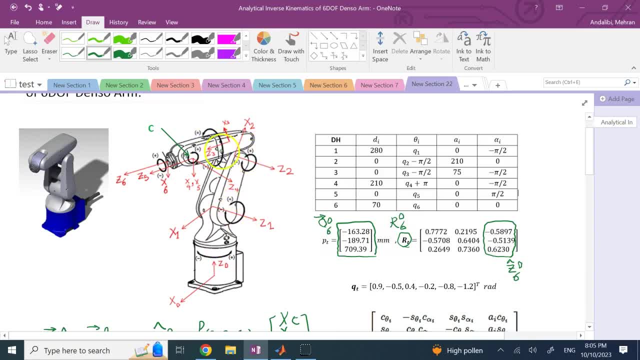 have theta 1 about this axis, theta 2 and theta 3, then theta 4, theta 5 and theta 6, and theta 4, 5 and 6, or these last three axes. they form a spherical wrist, basically. 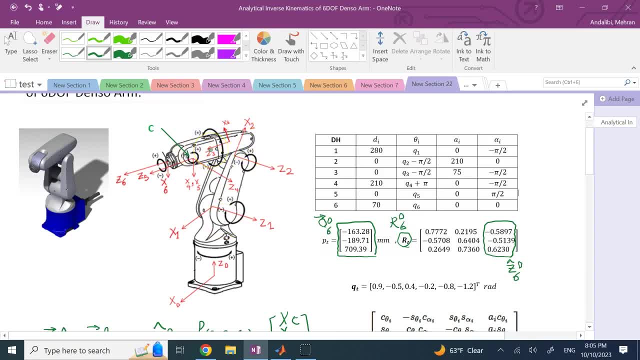 And since this robot has 60 OF and it has a spherical wrist, therefore we can solve analytical for the inverse kinematics problem. So if I give you a position and a rotation matrix for end effector in base like these two, So I say put the end effector at this. 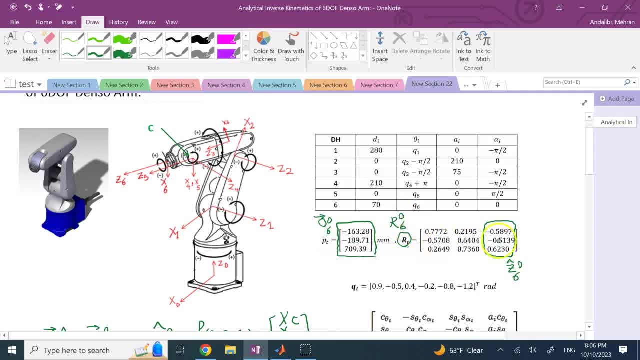 like these two. they cannot be rotated or rotated and of course, at some they cannot be rotated any more. If I gave a certains 6000 probability matrix of frame 6, which is end effector in frame 0, which is the base frame i want you to give me, 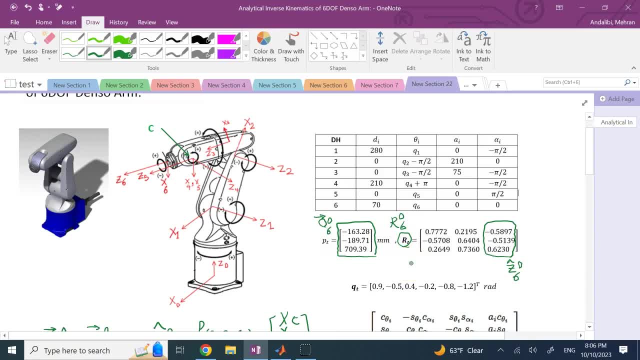 the joint variables q1 to q6. this is the answer, so i provided it. so when we go through the math lab code, we can see whether we converse this number or not. okay, so this is where we want to be, and these data are given, as well as the geometry of the robot, which is given with this dh table. 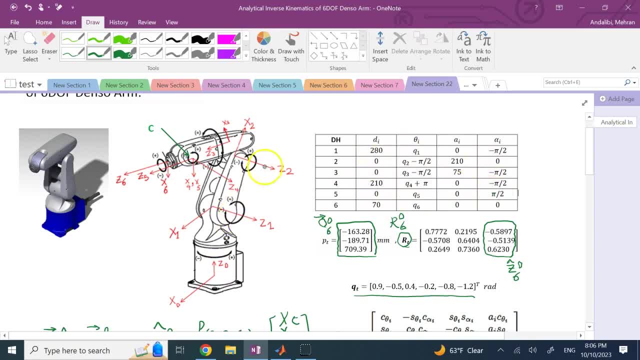 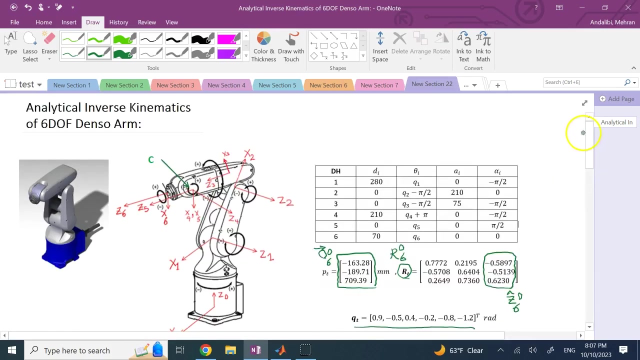 so this is the dh table for this robot. here the x's are shown on the robot, from frame 0 all the way to frame 6, and these are the parameters for the robot, the thetas, these a's and alphas. okay, for all of the six degrees of freedom. so now, if we want to solve the analytical problem, 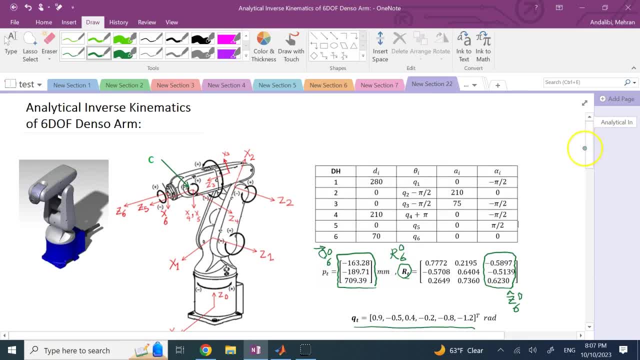 we're going to break that into two subsets. one is called the inverse position problem, the other one is called inverse orientation problem. and what is that? well, here i can tell you that if i call this point here, where the origin of frame four and five is this point, if i call it point c, that point c which we call it the center of the wrist, that 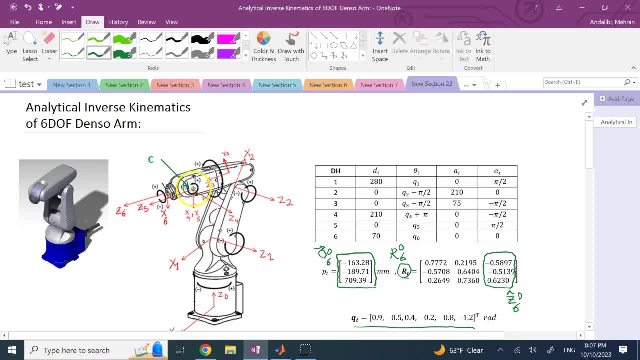 point. the position of it does only depend on theta 1, theta 2 and theta 3, this theta 4 here, this theta 4 or q4. this q4 has no role because it's rotating about this axis z3. it's not going to affect the position of this point c. so if i have the q1, which is here, q2, which is here, and 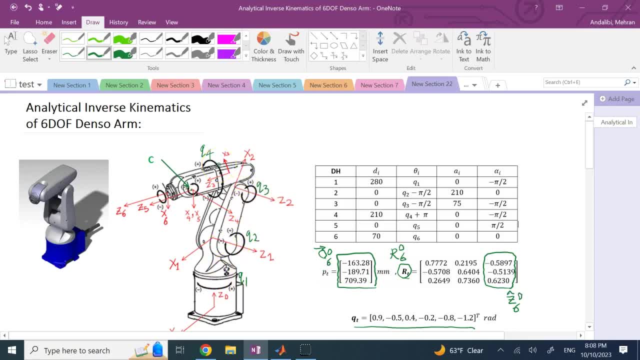 q3, which is here. if i have those, plus the first four rows of my ds table, then i can determine the location of c. and then you might say: well, you said only three qs. the first three qs are determining the location of c. why do you need four rows? well, the only thing i need from the fourth row, 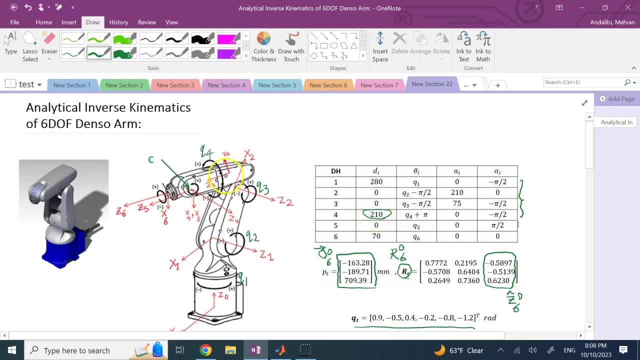 is actually this offset 210, which is the distance between origin three and two. so if i have the q3 which is here, q3, which is b, two and b, q3 is d, c, d, three and 3 is of the same length and the offset is 203, which is the distance between origin three and three. 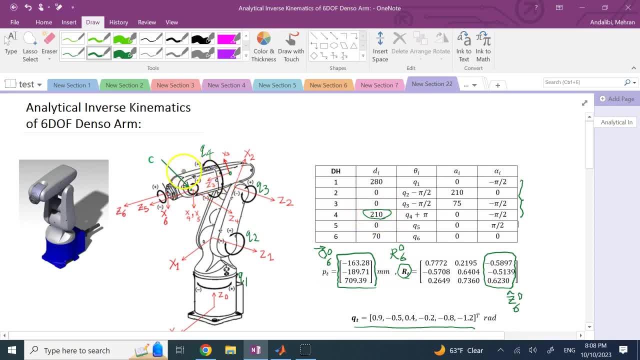 three and origin four. okay, so this offset from here to here, this offset, this one from here to here, this is 210. i need that offset because i'm calculating really the origin of four, not the origin of three. but again, this rotation q4 has no effect whatsoever on the position of this point. 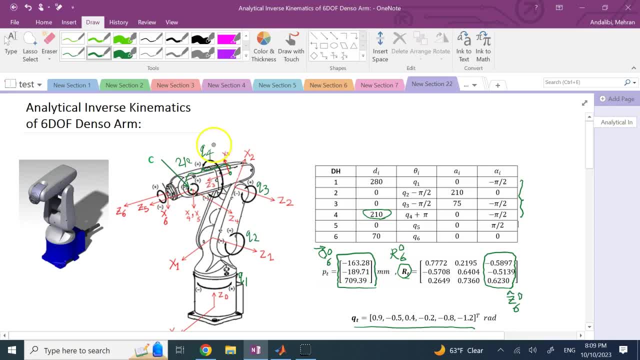 because it's about xz3. so this is what i do: first, i want to find the location of the center of wrist point c, and one way that i can find the location of this wrist is if i come back from this origin six, from the location of the end effector, which is this guy here, this given vector. if i come back, 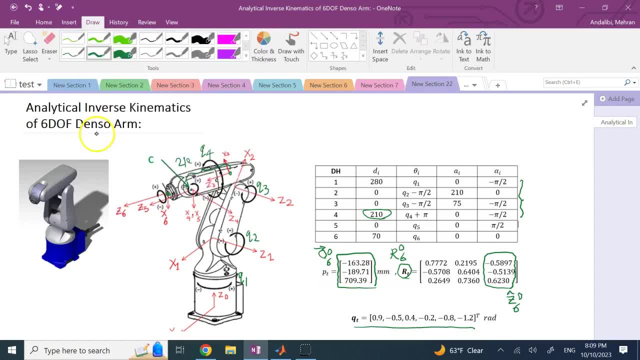 this offset. let me use a different color, maybe you can see it better. if i come back this much, just this much here, that's that, uh, that amount. if i come back that offset and in the direction of z6, if i come back that much, then i can get what i can get: the position of the wrist. so basically, basically. 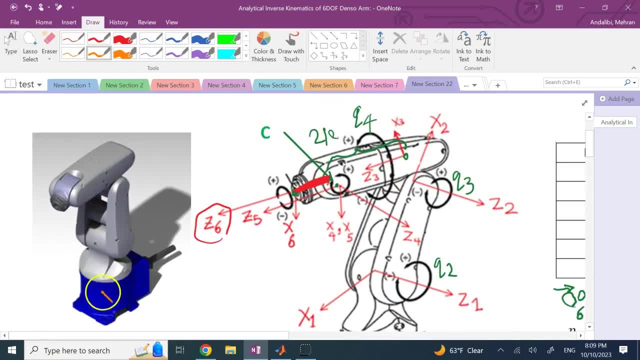 i have this vector. this is r of o, of sorry, origin of c and zero. i have this vector which has that offset and that is in the negative z жизнь direction. now of course you have to write the z6. uh, in terms of frame zero and the magnitude of this guy, if you look in the table. 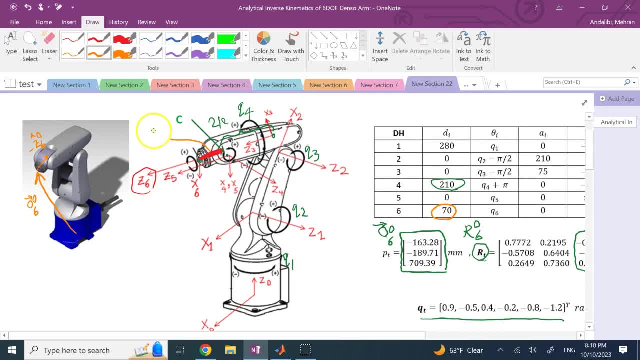 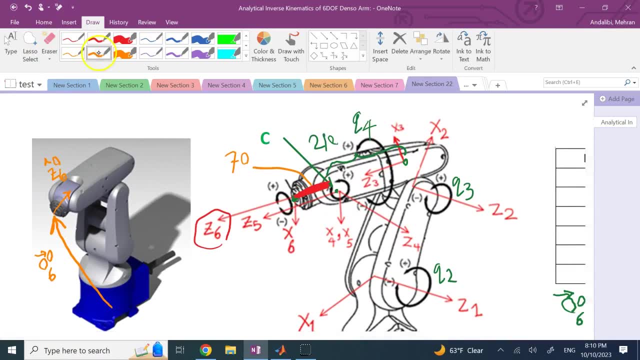 that is this number, 70. so that is what that is: 70. So if I come back negative 70, right and add it to this, then I can get this vector in red, which is the position of the wrist, and I can call it O of C in frame 0, right. 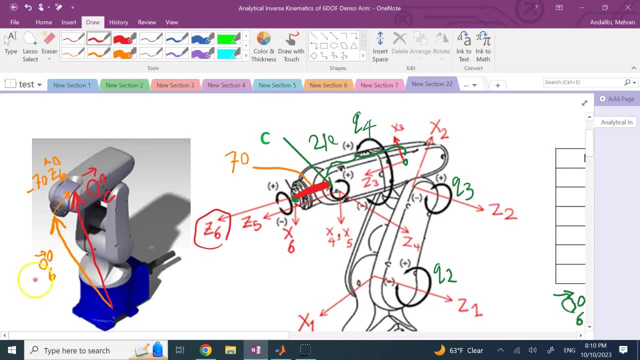 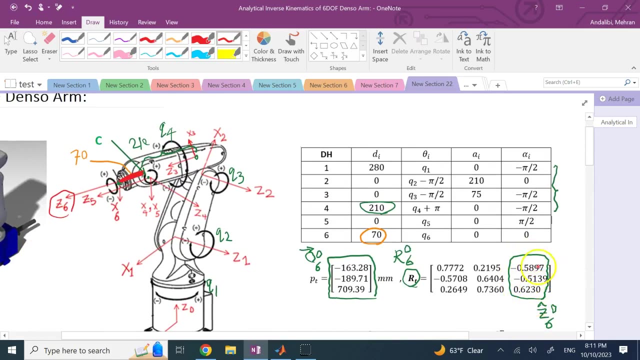 So if I add these two vectors- and they are all given because this position of the end of vector in base is given- this number 70 is given in the table and the Z of frame 6 in 0 is definitely what is the last column of the given rotation matrix R of 6 with respect to 0, the last column of it is Z of 6 in 0. 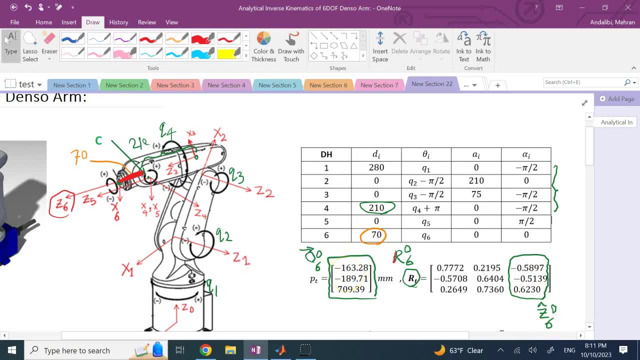 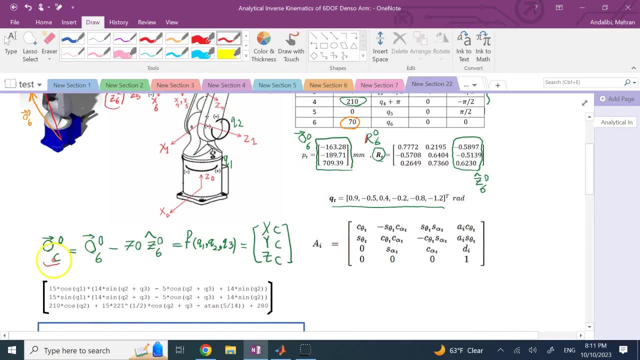 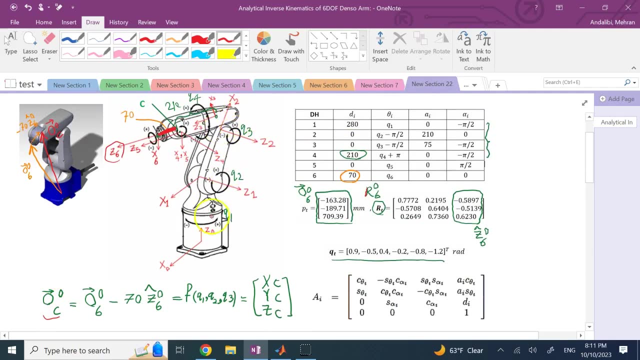 So I have that, I have this offset, I have this position. If I do that subtraction I just showed you, which you can see here, it gives me the position of the center of wrist in frame 0, and I can get it as a bunch of numbers and, as I told you, it's only a function of the first three joints. okay, right, 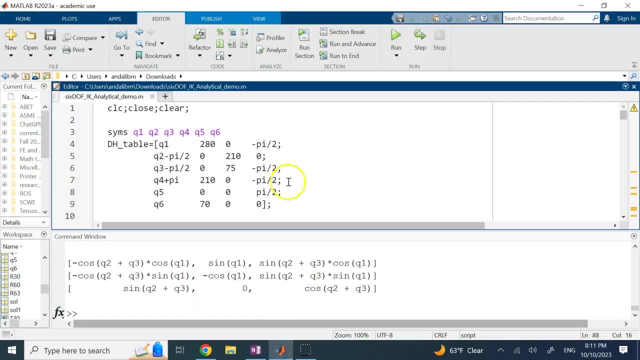 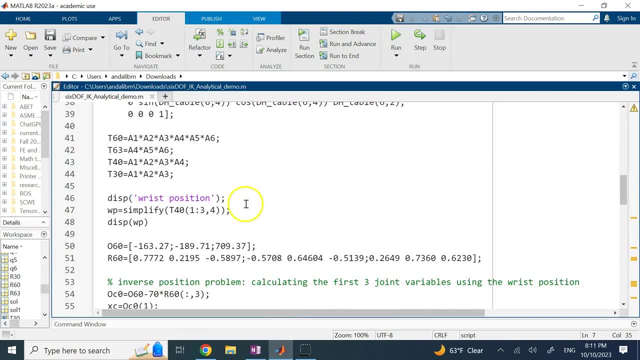 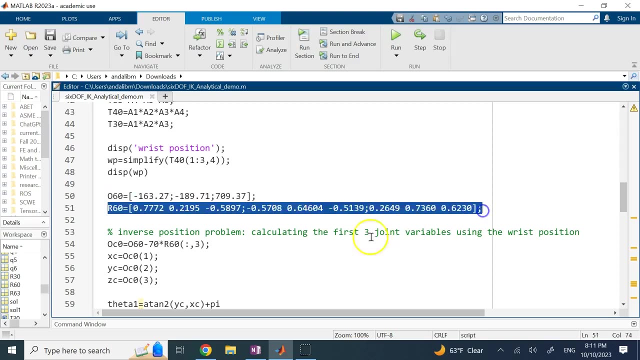 So here in Math Lab I want to show you that. So here I'll come back to these lines that I'm skipping. What I have is the target position for the end of vector and the target rotation matrix for the end of vector. 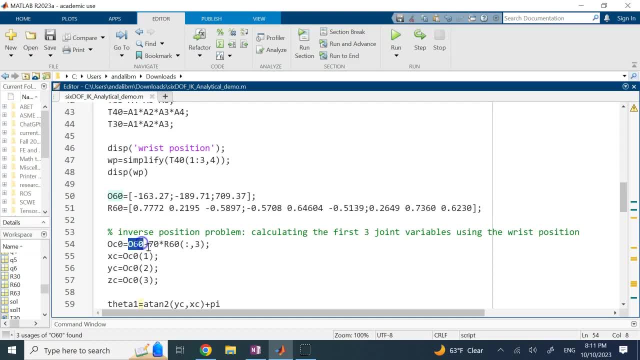 This is what you can see I'm doing. I'm subtracting the position of end of vector minus 70 times the third column of the rotation matrix, which is Z of 6 in 0, and I call it O of C in 0, and the components of that. I call them X, C, Y, C and Z C. okay, 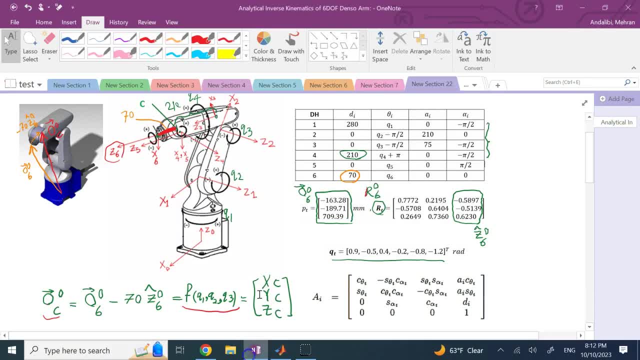 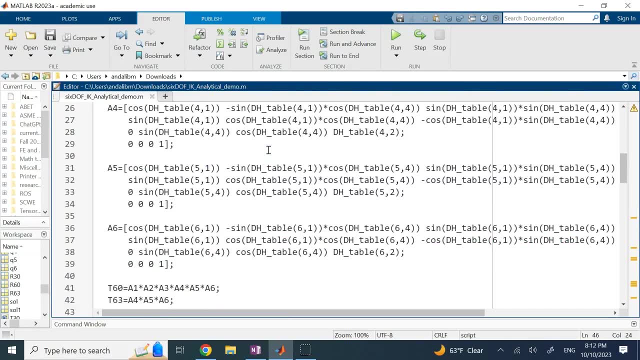 So these components are only X C, Y C and Z C. these are the notations I'm going to be using in my lecture. Now you might say: well, you told me it's just a function of the first three variables. 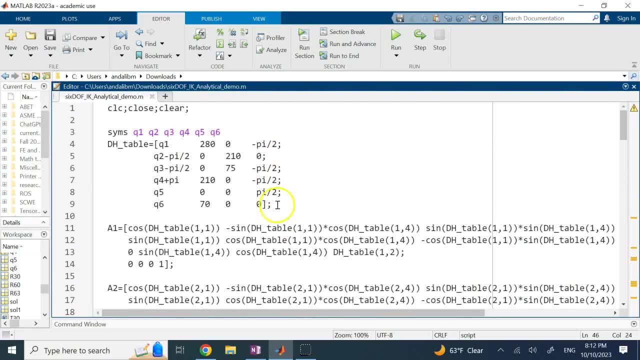 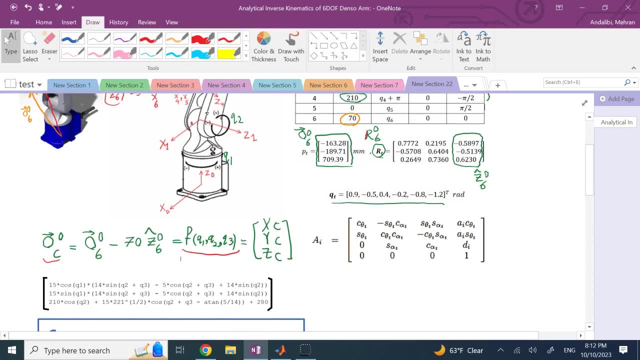 Can you show it to me in practice? Yes, So here this is that DH table I have, and then the A matrices for the DH. as you know, if we use the standard DH method, not the modified one, if you use the standard one, 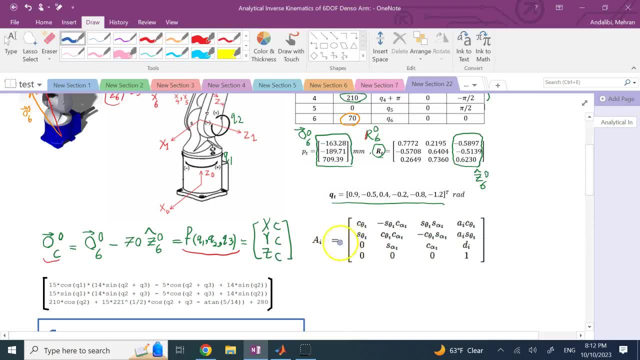 the A matrices, which are the homogenous matrices between frame I minus 1 and frame I AI, is this matrix So where these parameters, theta A, alpha and D, will be taken from the rows of the DH table? 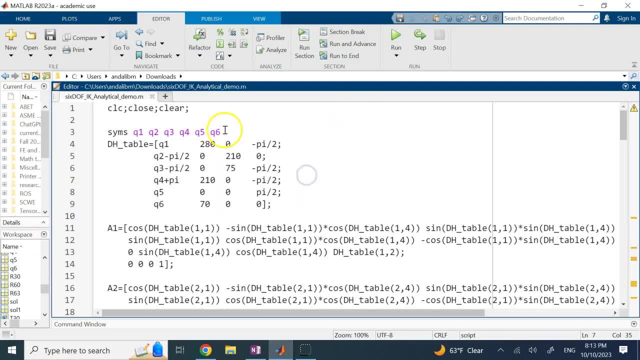 So that's exactly what you see I'm doing here, and doing it symbolically. So I define my six joint variables- Q1 to Q6, as symbolic, I form my DH table and then I plug in those numbers. 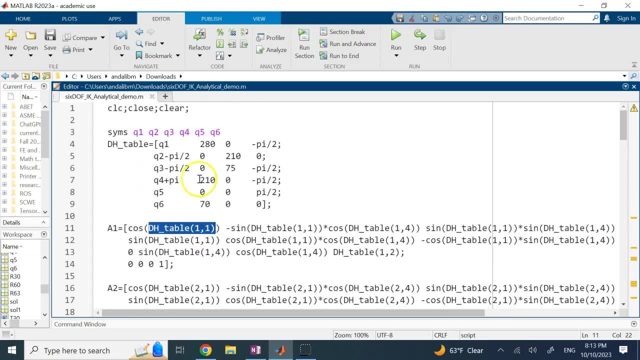 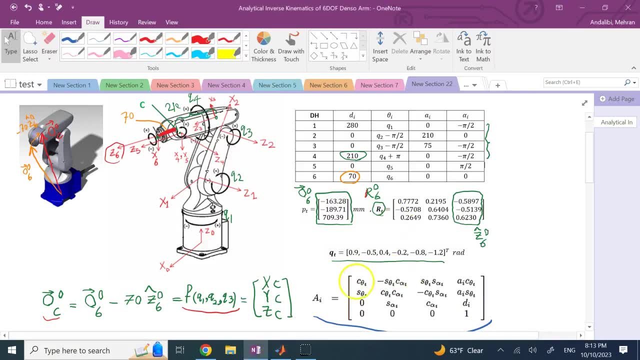 For example, I say DH, table 1 and 1, which is going to be what? Q1, that's cosine of that, and you can see here that the first element is what Cosine of theta, right, And so I form these A's: 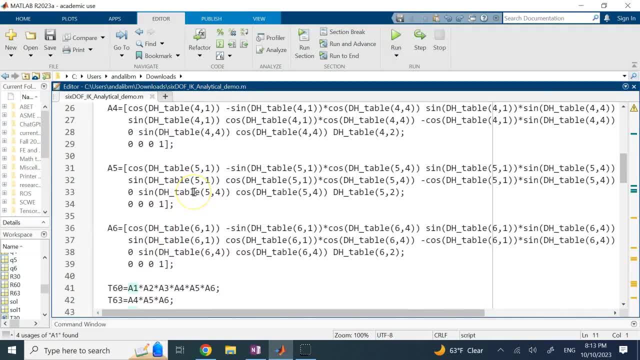 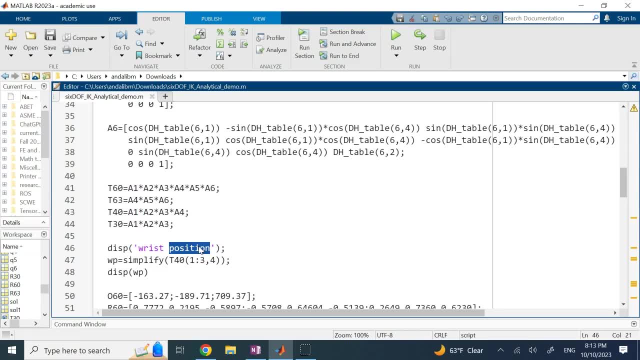 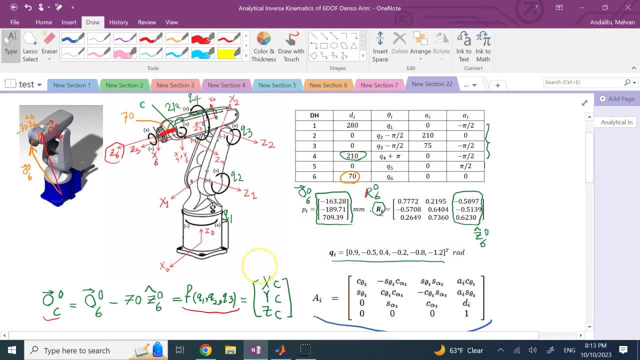 This is A1,, A2,, A3,, A4,, A5, and A6.. You can do it also with a four loop if you want. And now look, The wrist position, as I told you, is What is the position of the center or the origin of frame 4,, as you can see right. 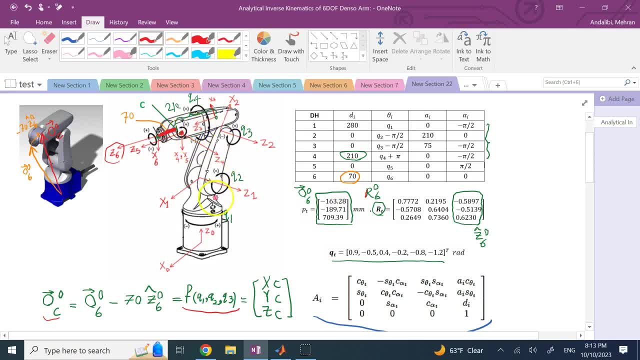 So if I want to get that as a function of all of the variables, it is the origin of frame 4.. So I need to what I need to use four rows. as I said, I need to multiply A1 to A2, to A3 and to A4.. 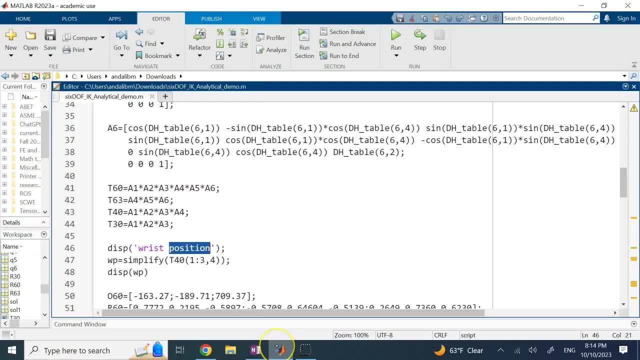 And get the position part of it, which is exactly what I'm doing here. So I multiply the first A's together. That's called T of 4 in 0, which determines the position and orientation of frame 4 in 0.. 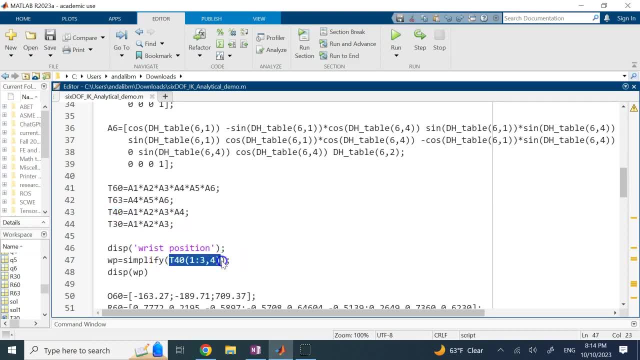 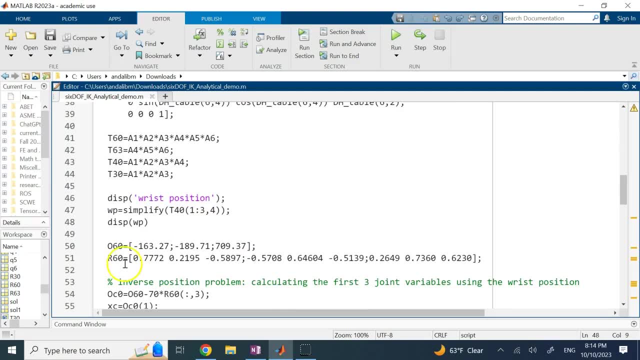 And then you see, I'm using what, I'm using the last column, the first number of it, which is the position, And I'm going to show it as what? As the wrist position. So look here, If I stop my calculations right here and I run my MATLAB, 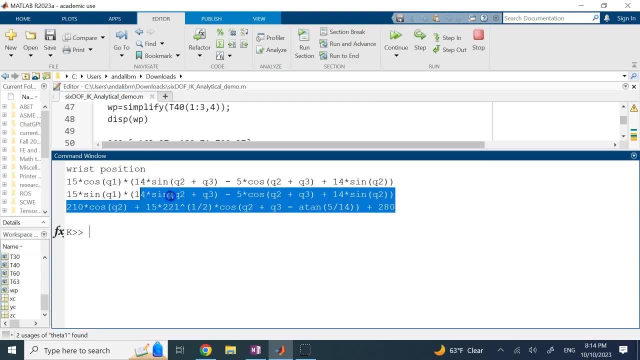 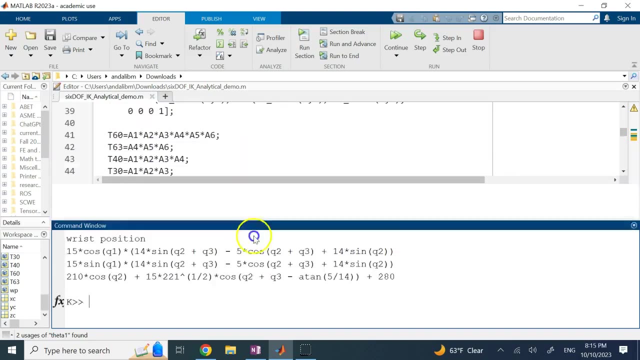 you can see that. look here: These are the X, C, Y, C and Z C as a functions of Q1, Q2, and Q3. And you see there is no Q4. Although in the definition, although here I'm using T40, and in T40 there is A4, and there should be Q4. 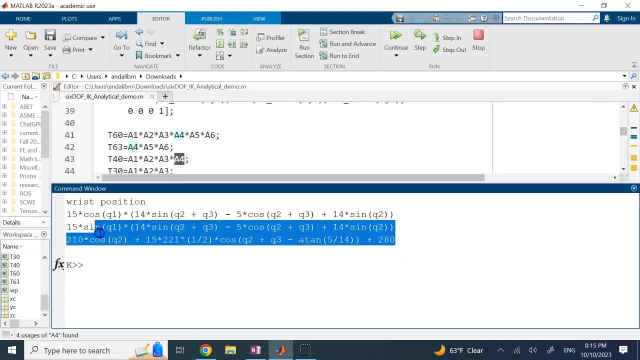 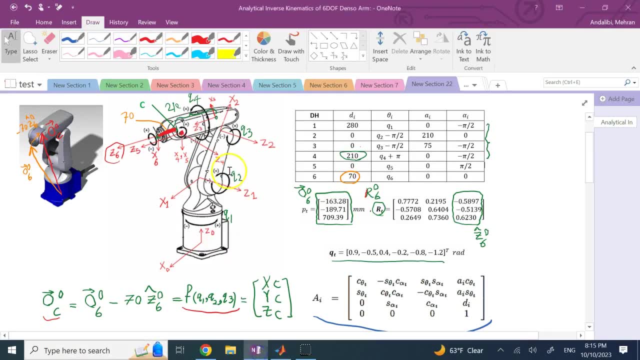 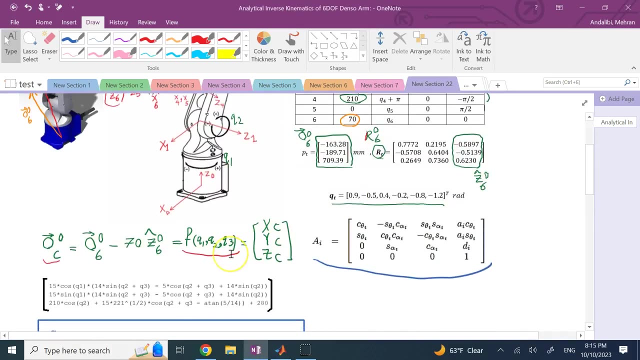 But you see, Q4 is not showing itself anywhere in X, C, Y, C and Z. So this part that the position of the wrist is determined only by the first joint variables And from there we can find the first joint variables. 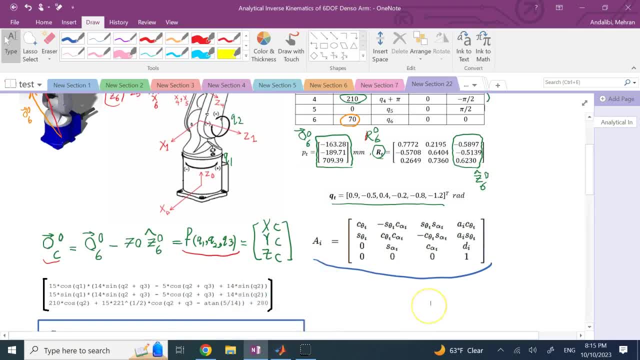 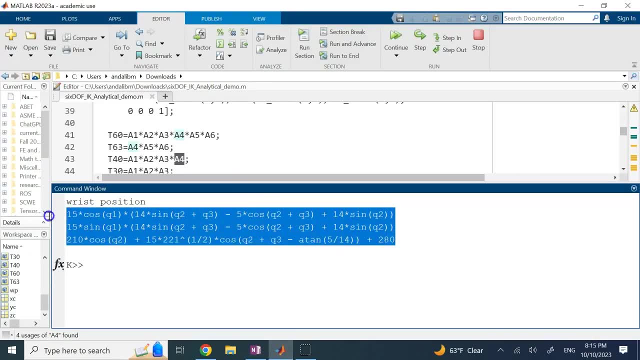 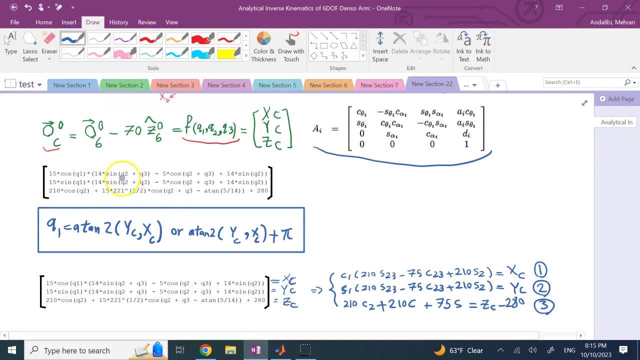 That part we call inverse position problem. So here, how do I do the inverse position problem? So here I copied these three equations into my notes Right here. These are those three functions: X, C, Y C and Z C. as you can see, 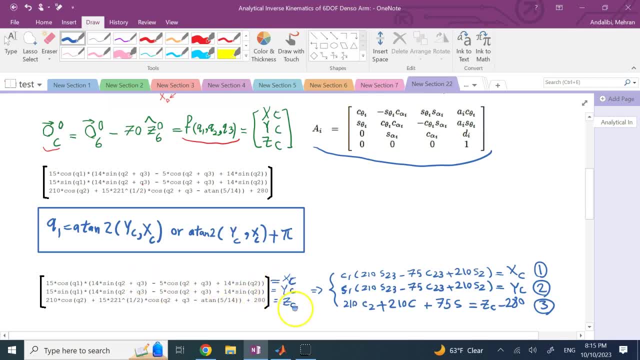 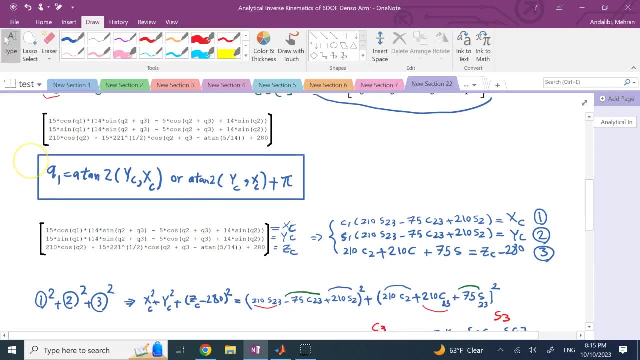 And my goal is to find what. Now I have three equations and three unknowns, Instead of six equations and six unknowns which I have for the 60OF robot. If you see, here I only have three equations and three unknowns. 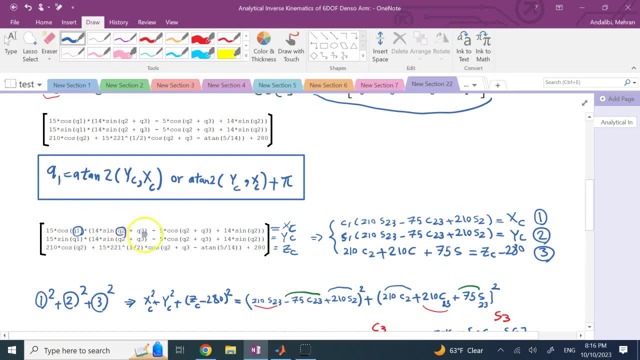 And the goal is to find what To find Q1, Q2, and Q3.. Now, how do I do that? Well, if you look at the first two equations, right off the bat, you can see that in the first two equations the same term here is multiplied to 15 cosine Q1 and 15 sine Q1. 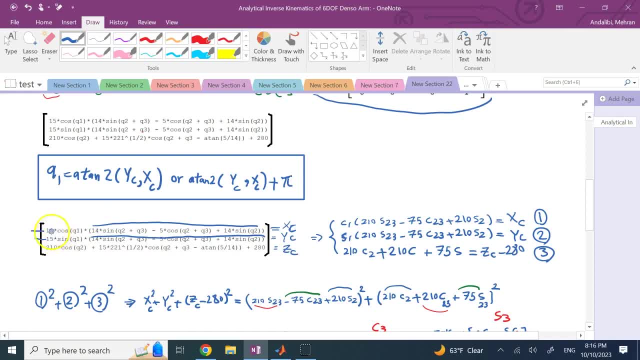 Since these are the same term, all I need is- and the 15 is the same- all I need is to literally pass Y C and X C because, you see, the ratio of Y C and X C is tangent of Q1.. 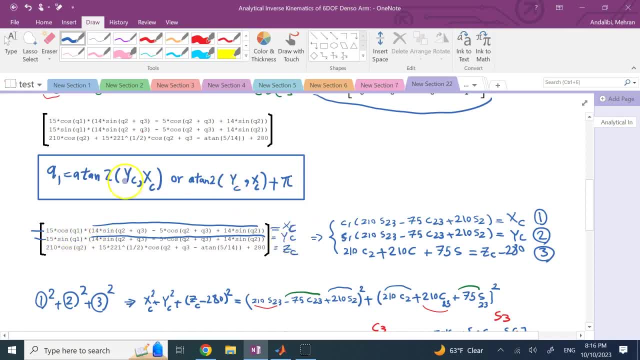 So if I pass Y C and X C to the arc tangent 2 function, that directly gives me what Q1.. That's one of the solutions. The other solution is to add 180 degrees to it, because you know, tangent of any angle and tangent of the angle plus 180 are the same. 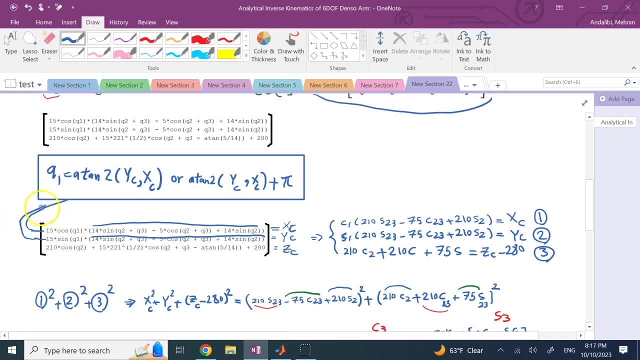 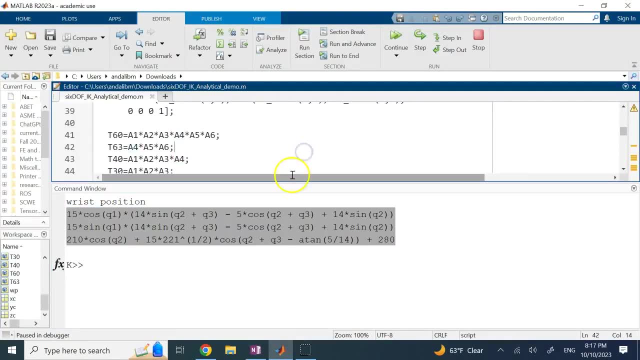 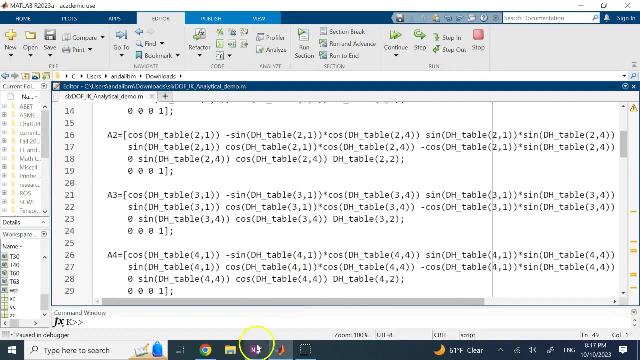 So here there are two possible. what Solutions for Q1,? as you can see Now, in this case the solution I have for theta 1 is the second one, So you have to add, Add a pi to it in this case, to get that desired solution here. 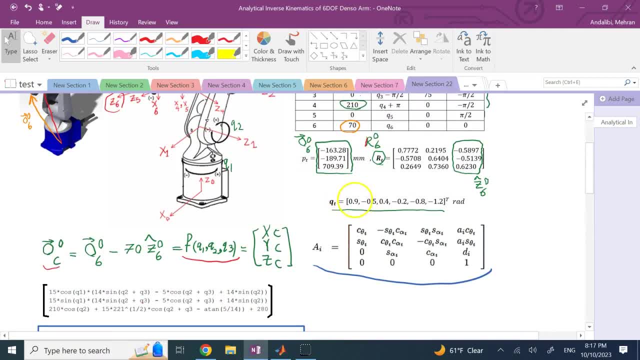 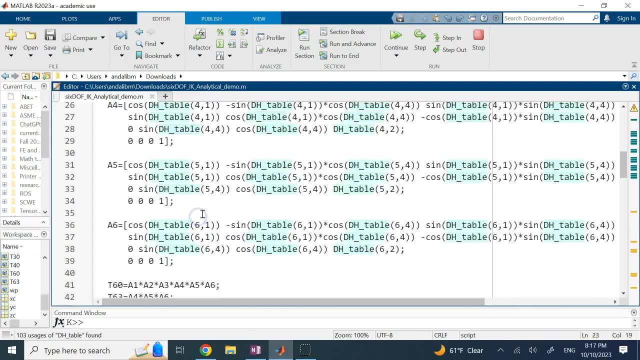 So if I want to get that 0.9, the first solution, Q1,, I need to use this second part, a tangent to Y C and X C plus pi, And that's what you can see I am doing here in the code. 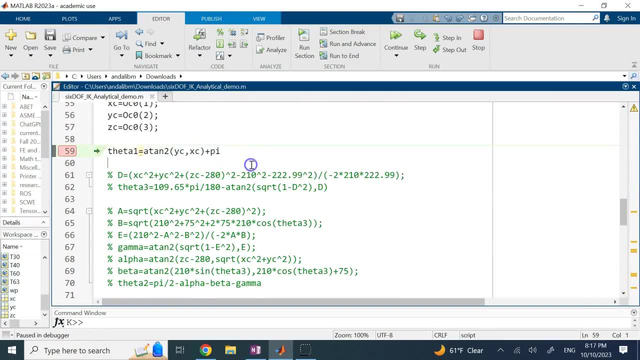 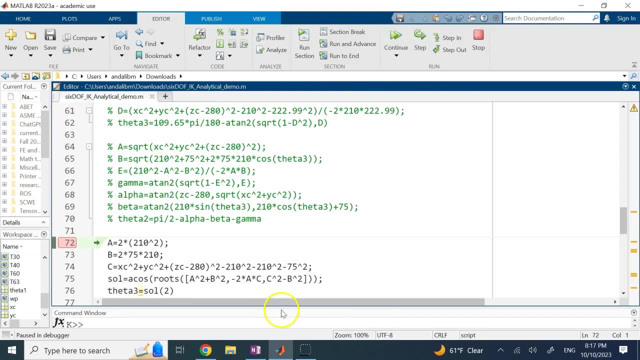 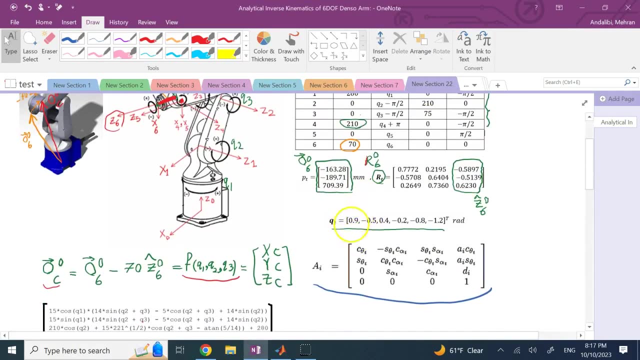 Okay, So I solve for what? For theta 1.. And if I do that here, okay, if I solve that for you, you can see that the number I get for theta 1 is what? 0.9, and that is exactly the number I have here: 0.9.. 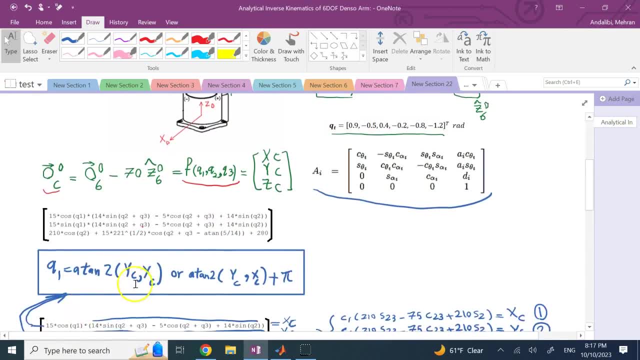 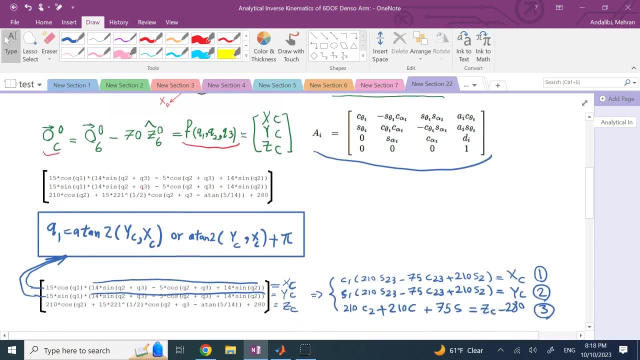 Okay, So I could solve for Q1 perfectly in terms of X C and Y C, which I got from this original equation. Now, what do I do? I go for Q2 and Q3.. Well, how do I go for Q2 and Q3?? 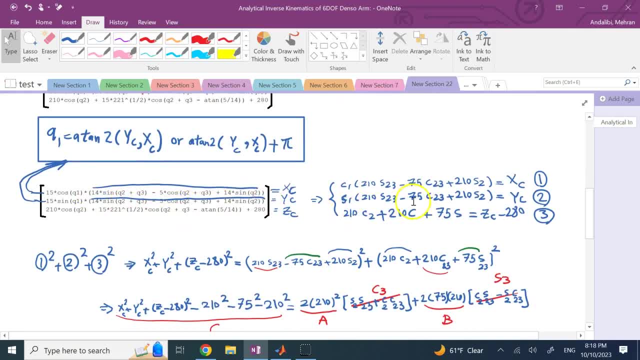 So here I expanded these equations And I used my notations here. where, for sine of Q2 plus Q3, I used S23.. And for cosine of Q2 plus Q3, I used what, C23.. Okay, These are the notations that I used in my previous videos. 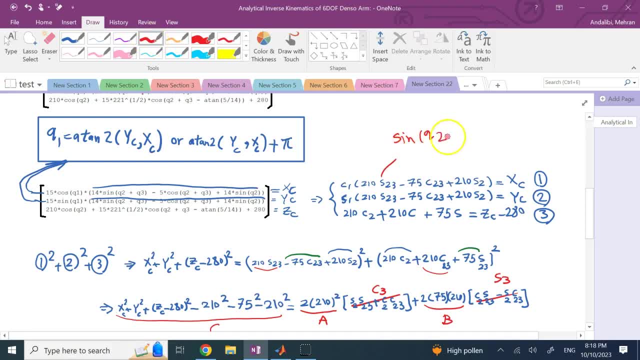 So this one is sine of Q2 plus what Q3. And this guy is cosine of Q2 plus Q3.. And also C1 means what It means cosine of Q1. And S1 means sine of Q1. 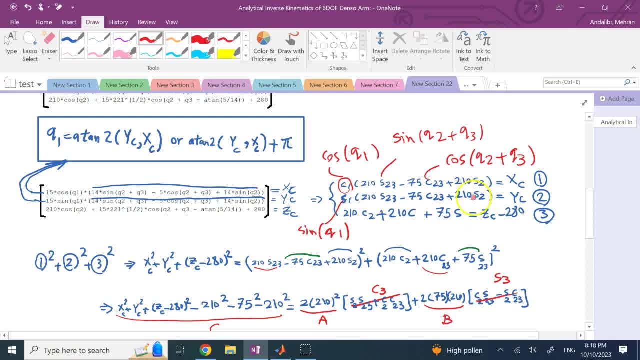 Okay, So here I'm using short notations so I can solve it faster. Okay Now, by the way, here there should be a 23 and a 23. Now that I know that I have expanded this cosine of Q2 plus 3.. 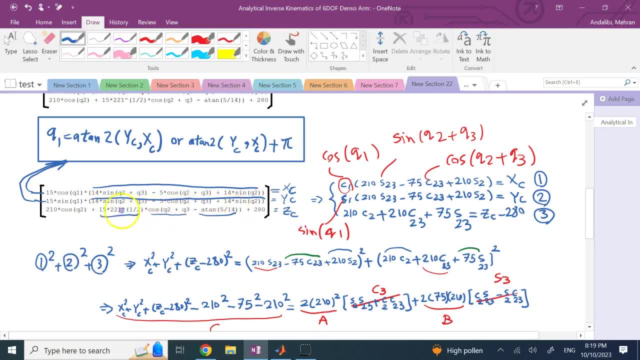 Minus arctangent. I expanded it, I expanded this term And I rewrote it as these equations 1,, 2, and 3, as you can see Now from these equations 1,, 2, and 3, the goal is what? 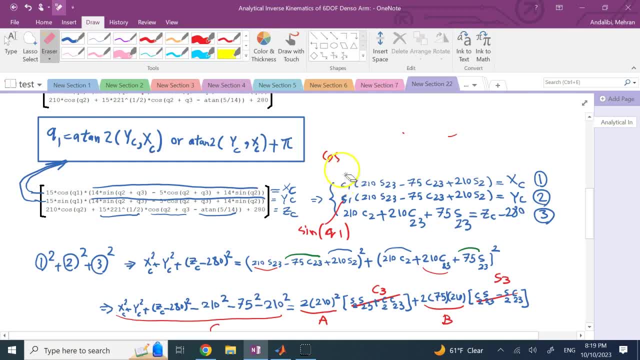 The goal is to solve for Q2 and Q3.. How do I do that? Well, I S-square equation 1 and 2 and 3 and add them all together. By the way, I brought this 280 to the right side. 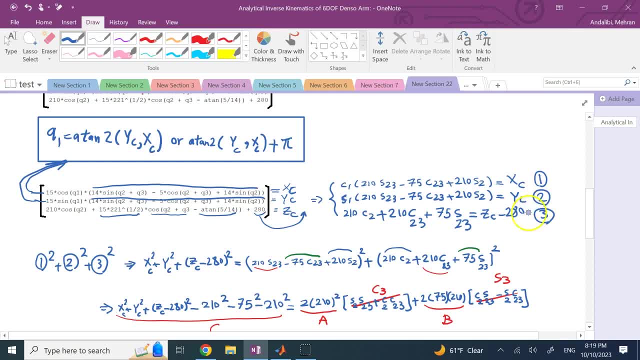 So it became negative 280.. Okay, So I square them and add them together. If I do that and simplify, do a little bit of algebra, since these two terms are the same, and you get cosine 1 squared plus sine 1 squared, which is 1.. 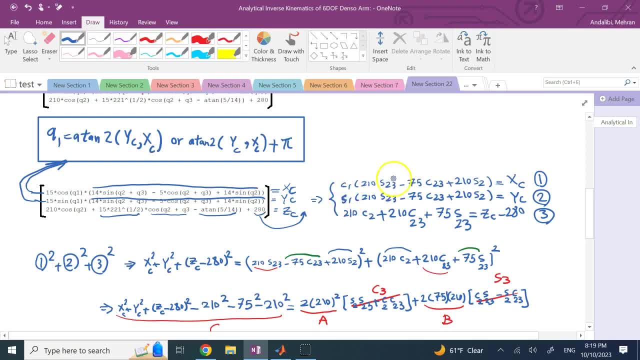 So the Q1 term would be eliminated. So you only have basically this term squared And then you're going to have this guy squared equals to XC squared plus YC squared plus ZC minus 280 squared, which is exactly. 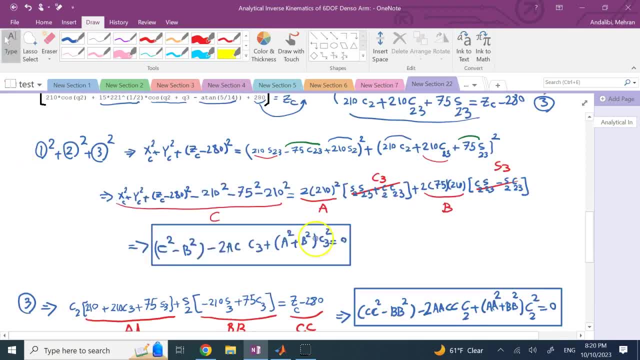 What you can see in the first line. Then here I have similar terms. So the terms in red they have the same coefficient, but they are S23 and C23.. The terms in green, they are similar: 75, C23, again S23. 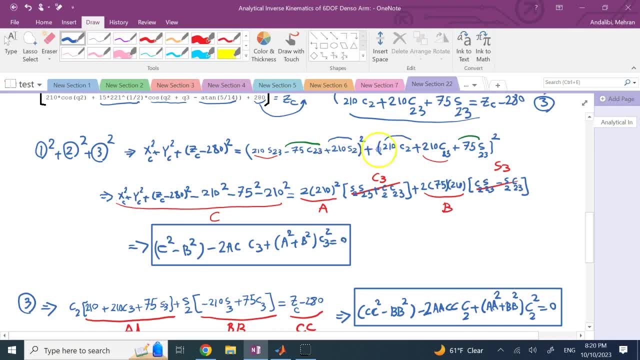 And the terms under blue. they are S2 and C2, with the same coefficient 210.. So when I expand, when I square each one of them and simplify, the sum of the two red terms squared just becomes 210 squared, which you can see here: 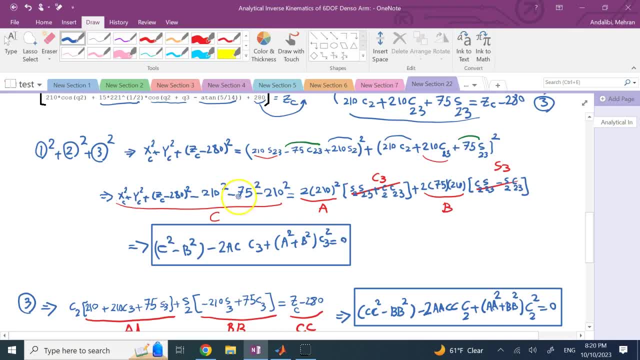 The sum of the two green terms squared becomes 75 squared. The sum of the two blue terms squared becomes 210 squared. And then I bring those constants- those 210s and the 75, instead of the right-hand side I bring them to the left-hand side and they all become negative. 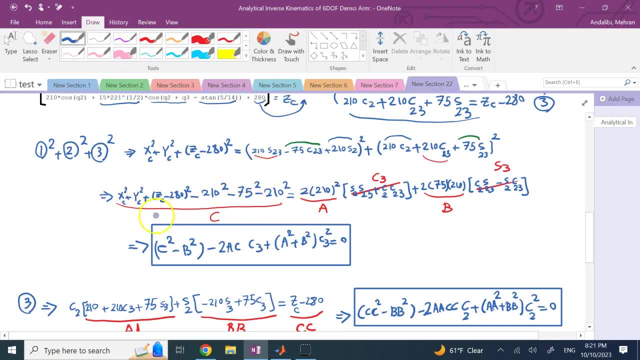 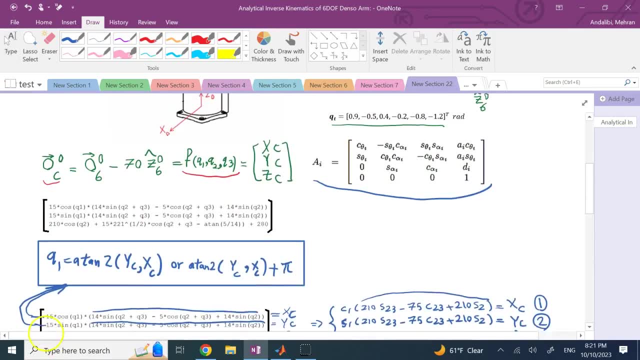 Why do I do that? Because now, if you look at my left-hand side, it's just a bunch of numbers. I know my X of the center, I know Y of the center, I know Z of the center. I already calculated all of them here. 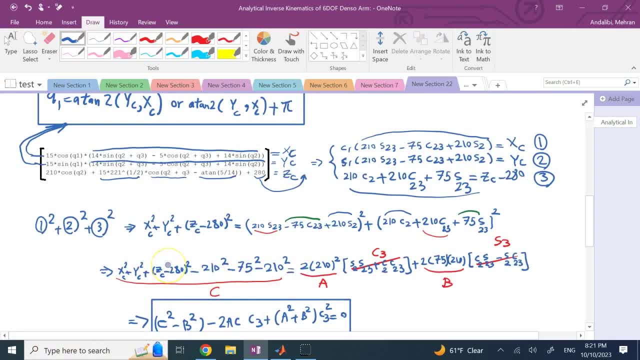 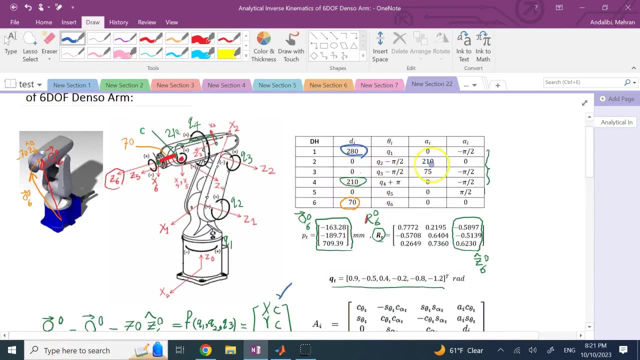 And these are all just dimensions of the robot, right? These 210,, 75,, 210, and 280,. you can see them in here, right, Look at them here. These numbers in blue are those numbers I'm using. 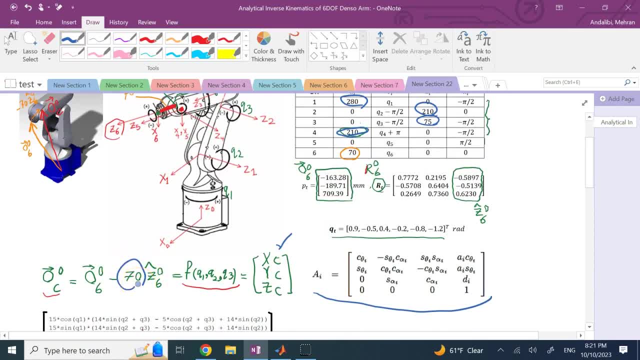 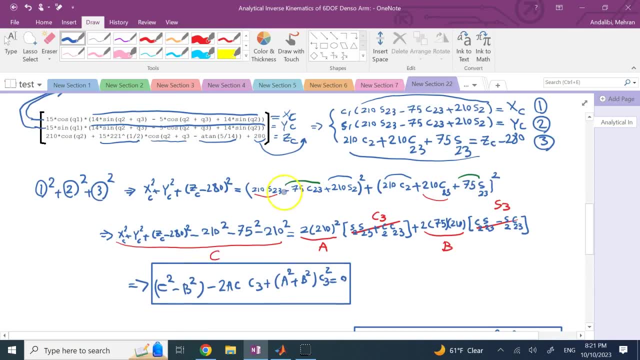 This one in orange? is this guy here? Okay, So you see, All of the geometry is being used here. And then the other terms that you have, like 2AB, 2AC, 2BC- two of them will be simplified. 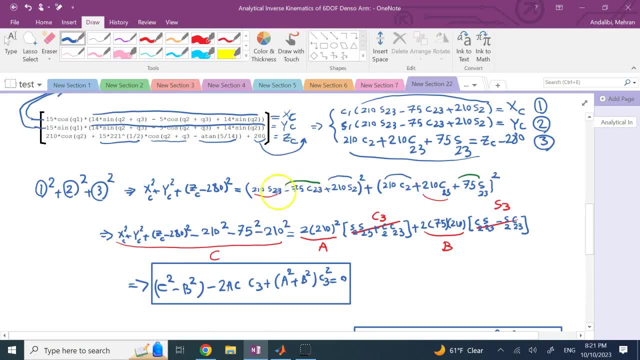 because there are like positive and negative right. This one is like negative S23, C23.. This is like positive S23, C23, and they would cancel each other And the four terms instead of the six terms would remain. 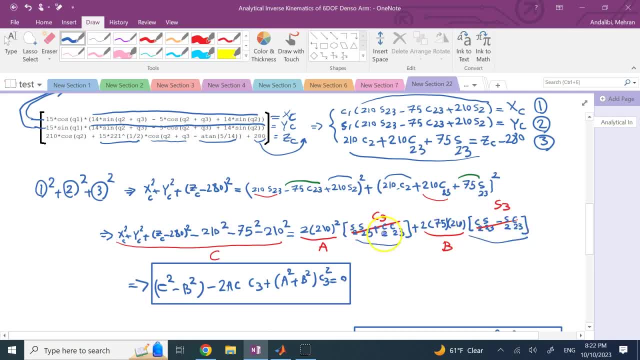 One of them is this guy, One of them is this one. And if you know trigonometry, simplify this: S2, S23, plus C2, C23.. That's cosine of 2, 3, minus 2.. 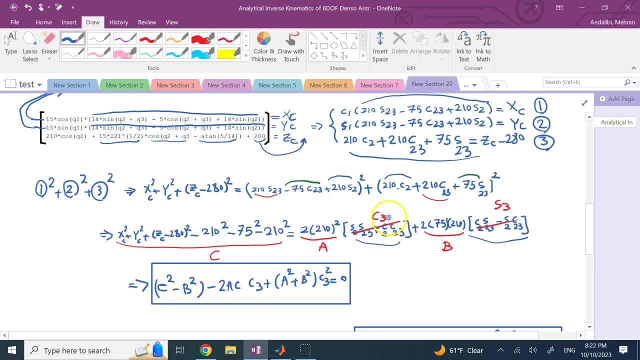 And cosine of 2, 3, minus 2 is just going to be cosine of 3.. And this one: C2, S23, minus S2, C23, that's sine of 2, 3, minus 2,. 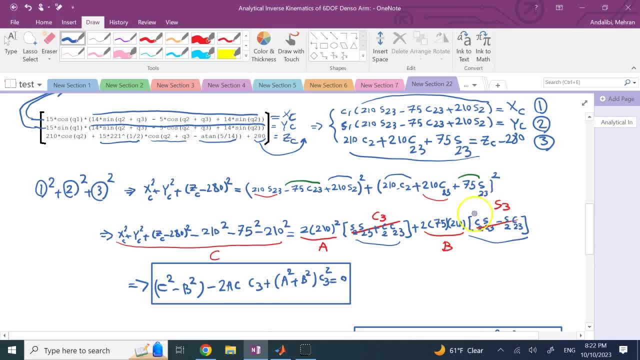 which is just going to be sine 3.. So my equation, if you give names to these constants, my equation becomes: A sine A cosine. So my equation becomes: B sine of theta 3, plus B sine of theta 3, equals C. 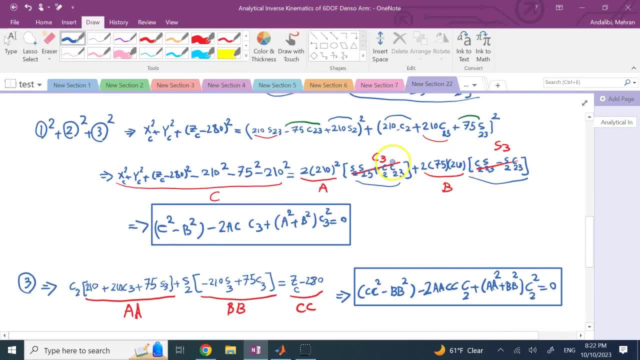 And A, B and C are just numbers And you can easily, by rewriting sine in terms of cosine right, writing this sine as square root, 1 minus cosine squared, you can convert this equation into a quadratic equation which you can see over here. 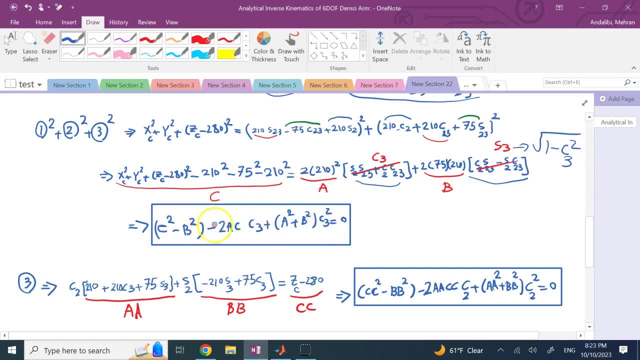 So now it's going to be this quadratic equation in terms of cosine of 3.. And so it's a polynomial with constant coefficients. So we can use the command roots In MATLAB and by giving it the constants this one, this one and this one. 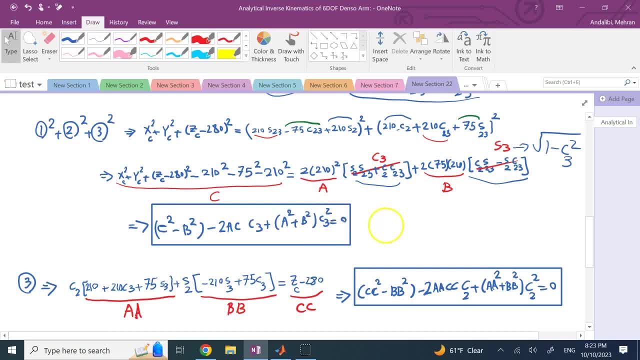 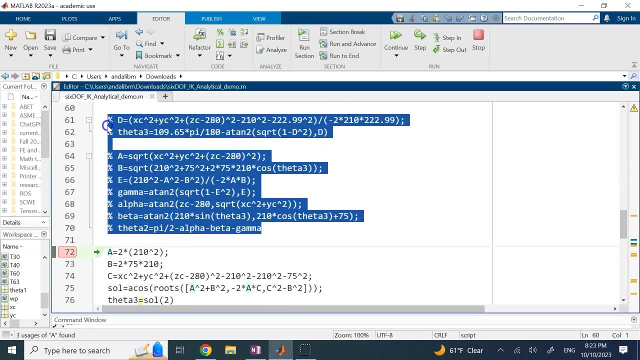 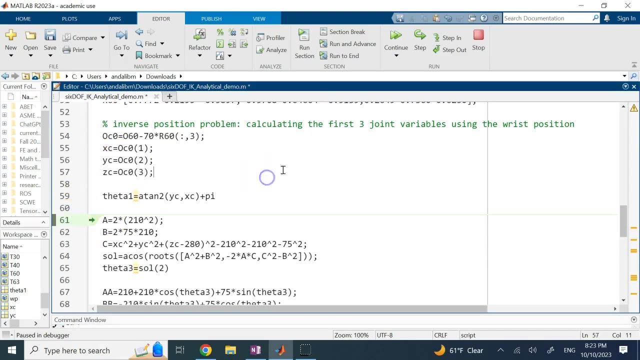 you should be able to find what C3, cosine of theta 3.. And this is what I'm doing over here. If you look at my notes, let me get rid of this alternative solution. Just go over here. So here you can see that I'm calculating A, I'm calculating B. 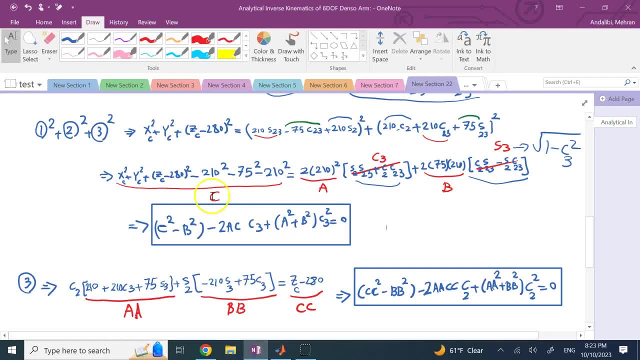 and I'm calculating C Just based on the definitions here I have for them. Then I go with the roots of this guy. The coefficient of the quadratic term is A squared plus B squared. The coefficient of the linear term is negative, 2AC. 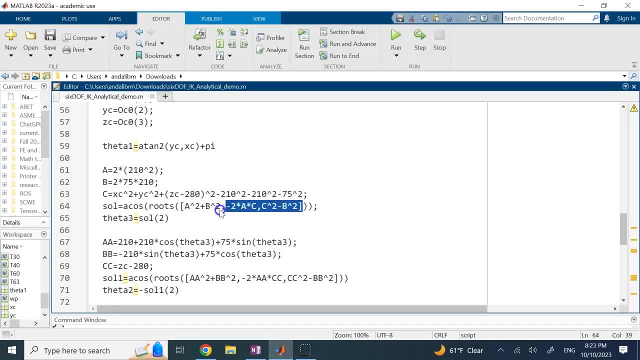 and the constant term is C squared minus B squared. So you can see, here I form a vector with those three numbers, I use the command roots And then that is cosine of theta 3.. Then I take a cosine inverse and I get my. what solution? 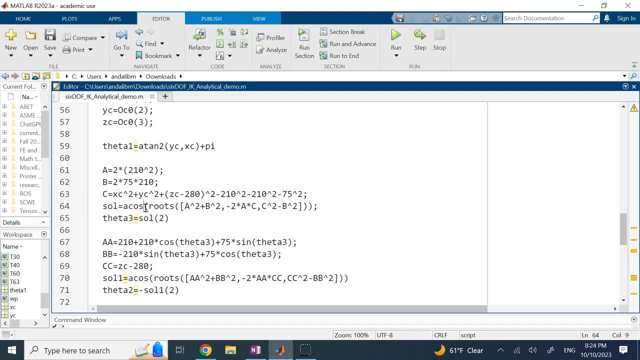 Now, if you want to use arctangent, you can do that. That's also fine. So you can call this one something right, Because that's cosine of theta 3.. So you can if you want to use the arctangent 2 command instead of that. 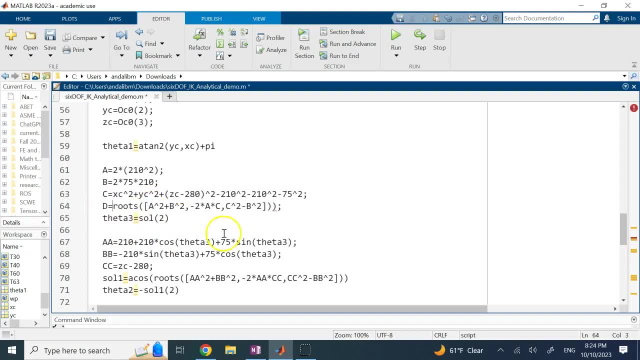 you can go ahead and call this, for example, D, right, You can call this D. And then you can use what Arctangent 2 of square root of 1 minus D squared, And what And D, And that should do the job for you, right. 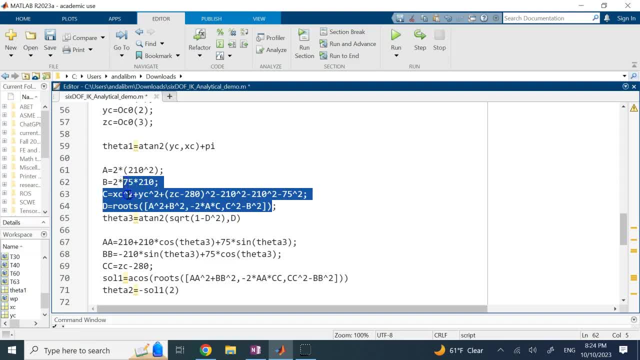 So if I go ahead and look at D right now, Now D, the thing is, it has two roots And here we're going to just use one of them. So look here. If I go ahead and look at the solution, let me run this part for you. 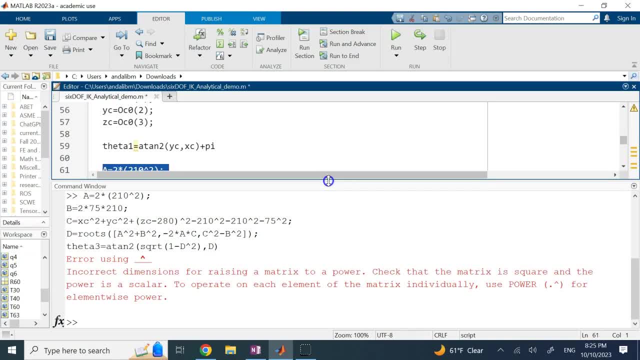 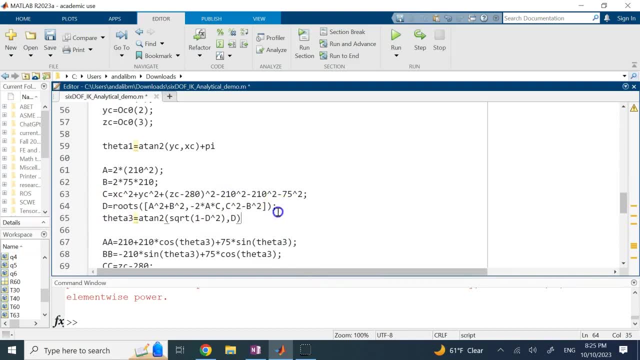 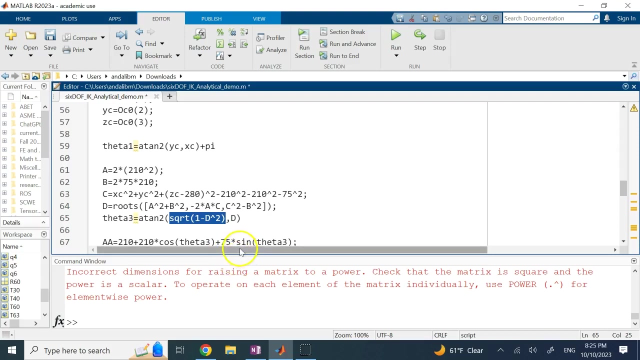 Oh, seems like I got an error. Okay, let's look at the D. D is the root. Let's look how much the D is. So there are two solutions for D, right, And then this one here should be. you can see I have an error. 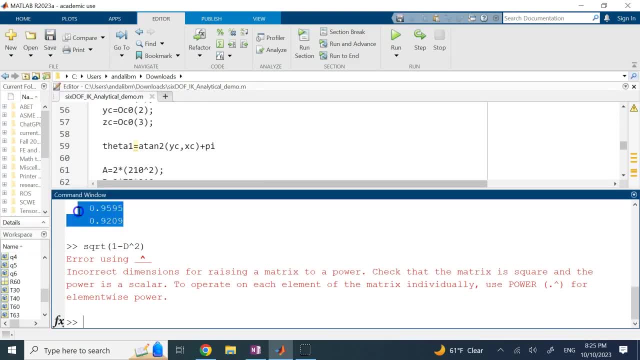 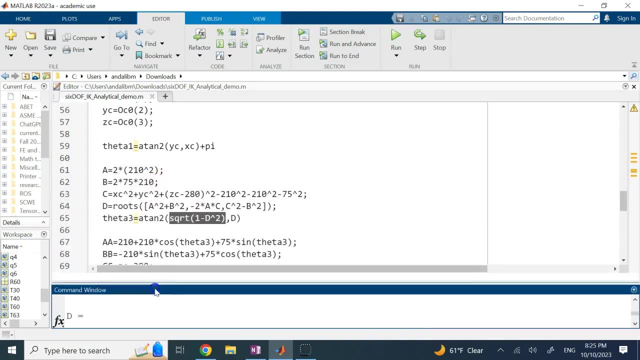 Raising a matrix to a power. ah yeah, Because here I have two solutions for D, So I need to only Go with one of them, Either D1 or D2.. So here, let's say, I just go with D1.. 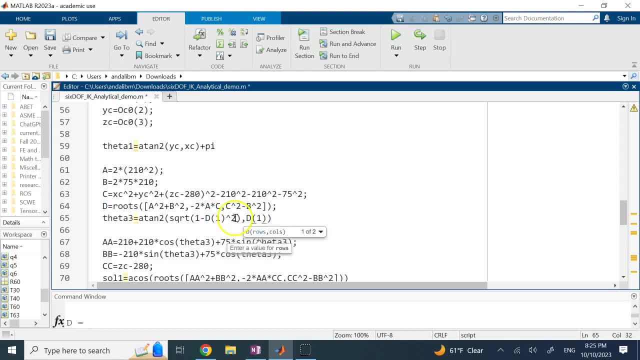 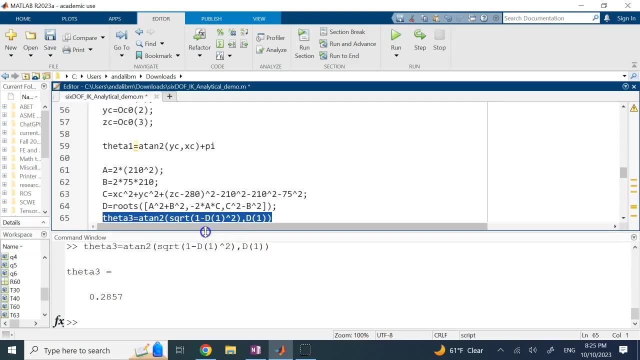 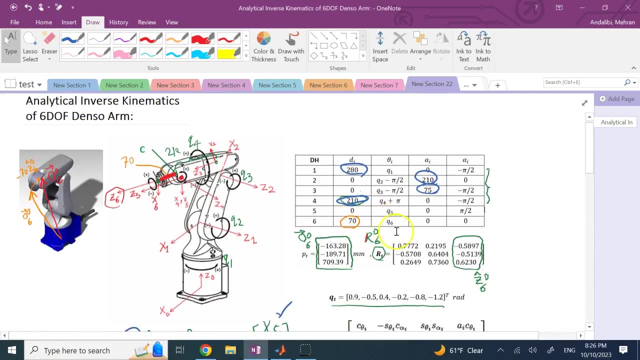 And see what happens, Whether I get the answer in the node or not, Or I need to use the other solution. So you see, theta 3 becomes 0.2857.. While the solution here is basically 0.4, as you can see. 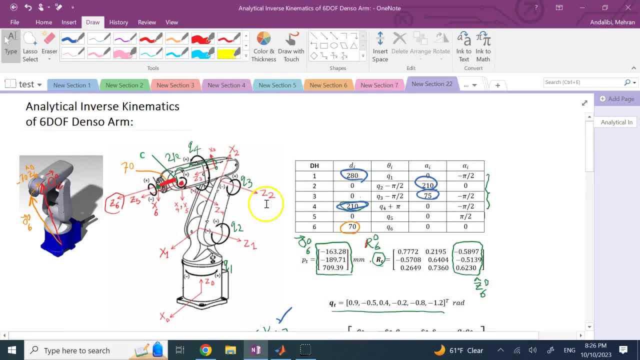 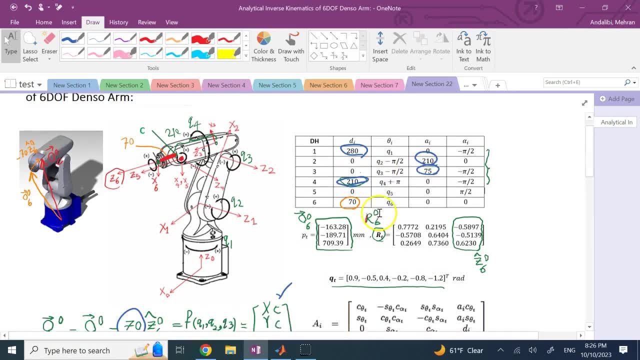 But remember that This robot, this Denso robot, has 16 different solutions. okay, The inverse kinematics problem, for this in general, has 16 different solutions. So there is a chance that the one that we got with D1 is not the solution. 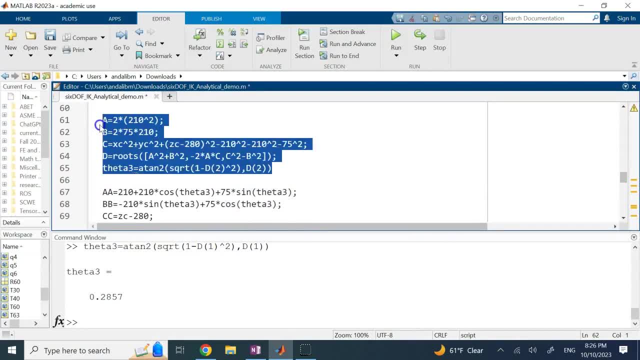 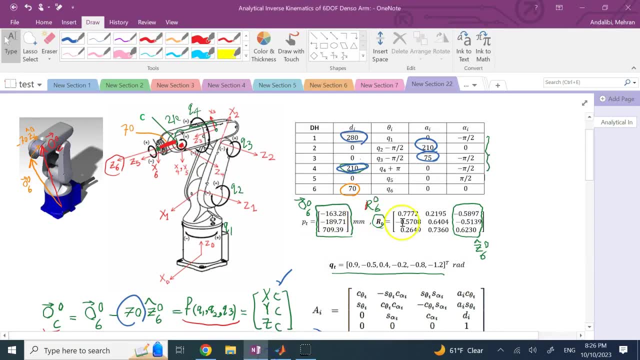 So here the desired solution. if I tried with D2, let's find out, There we go. Look, it's 0.00.4, and that is exactly this number I wanted. Okay, So you see, I got my what. 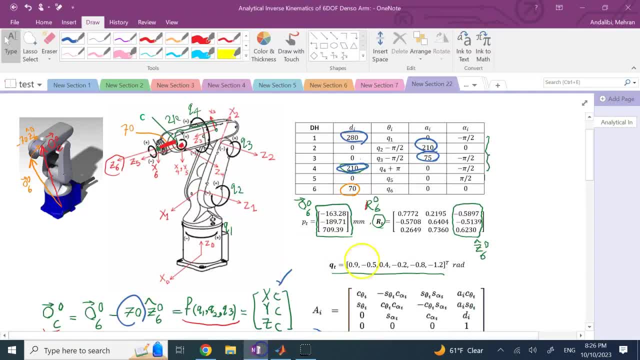 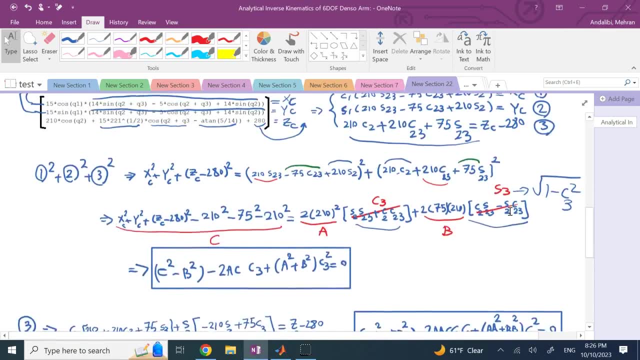 I got my theta 3.. Now that I have my theta 3, let's go to theta 2.. So, for theta 2, what I'll do? I'll expand the last line, This equation 3, I expand it. 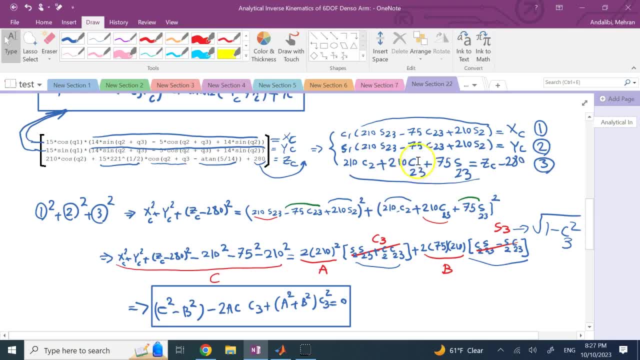 I expand cosine 2, 3.. You know, cosine 2, 3,, which is 2 plus 3, is going to be cosine 2,, cosine 3, plus, minus, sorry, minus- sine 2,, sine 3.. 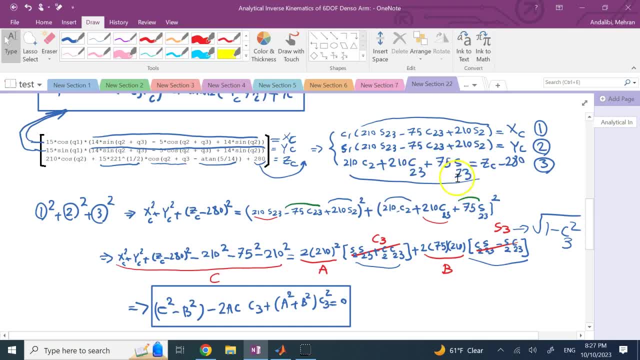 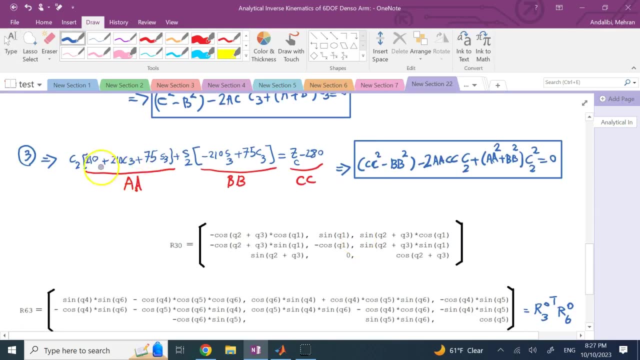 And this one, S2, 3, is going to be sine 2, cosine 3, plus cosine 2, sine 3.. And then 3 is now a known value. Theta 3 is a known value. So what I did? I have rewritten equation 3 in terms of the knowns and unknowns. 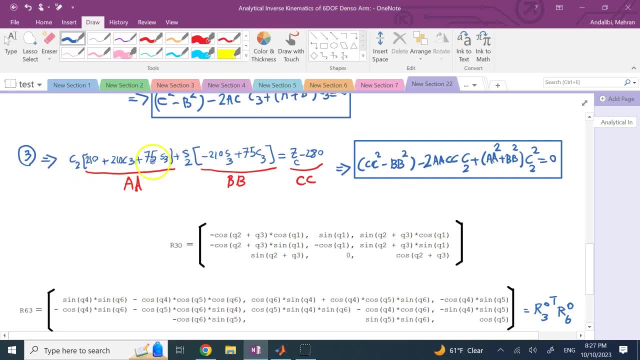 So I factor out C2 and S2, which I don't know, them, and then everything else which I know, including theta 3 and sine and cosine of that. I wrote them inside, I factored them, I factored them out. 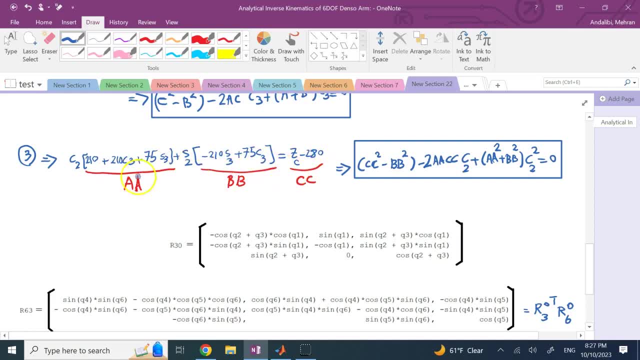 Okay, And the right-hand side is also a known number. So if these coefficients that I underlined for you- a, a, b, b and c, c- these are all just a bunch of numbers right now, because I know theta 3.. 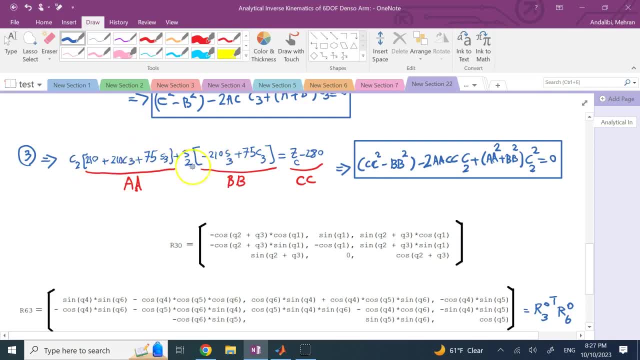 Again this equation here: something times cosine of theta 2 plus something times sine of theta 2 equals. another thing can be written in terms of what A quadratic equation in terms of cosine of theta 2.. The exact same thing that we did for theta 3.. 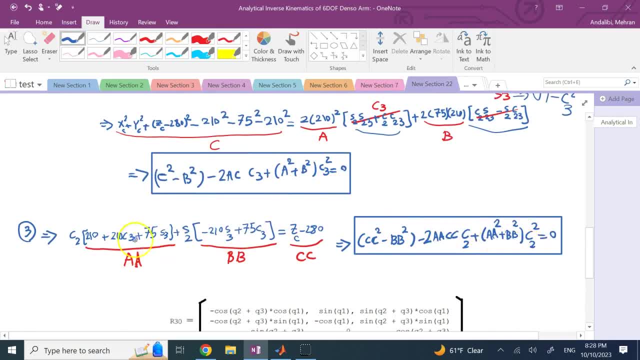 We can do it for theta 2, but with these new coefficients a, a, b, b and c, c, And again that gives us cosine of theta 2, from which we can find sine of theta 2, and then theta 2 itself. 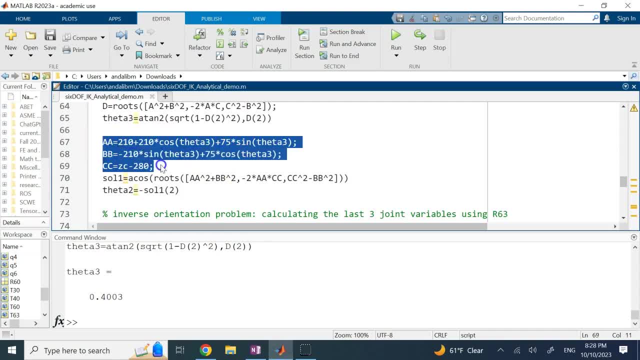 Okay, So here you see, I define a, a, b, b and c, c, exactly based on those coefficients. And again, if you don't want to use the r cosine, which is not really a good idea, maybe this time call this one: d, d. 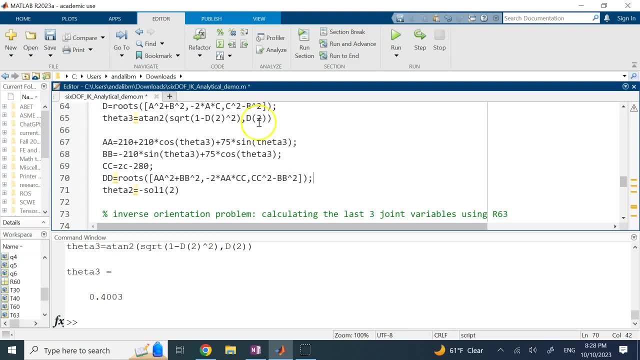 And um, This is just going to be the roots of that. and then theta 2 is going to be: what An arc tangent function. And here we have to use d d, and it might be d d 1 or d d 2.. 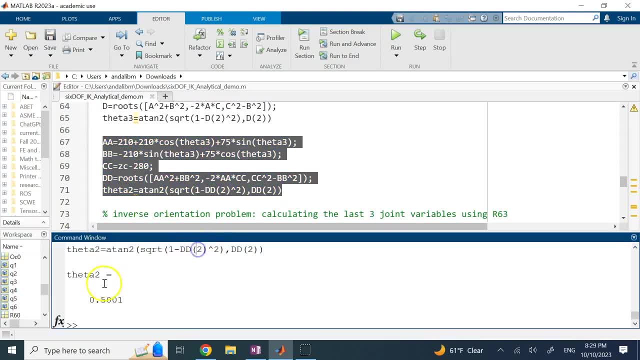 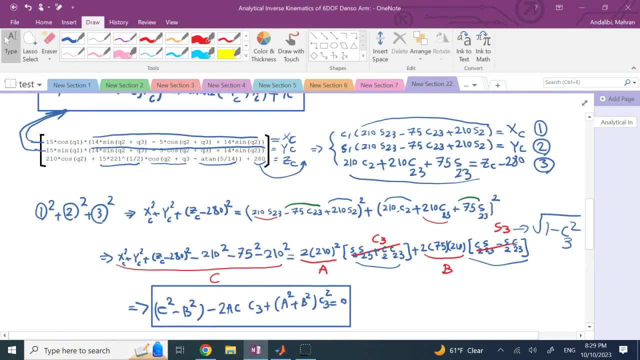 So let me calculate that one, and there we go, You see, with d, d, 2, the answer is what? 0.5.. And in this case, if we look at the solution, the answer is 0.5.. 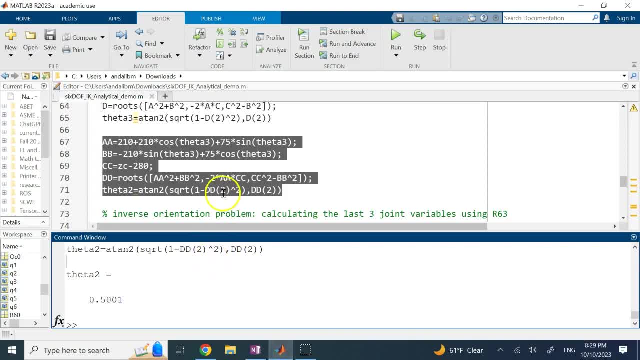 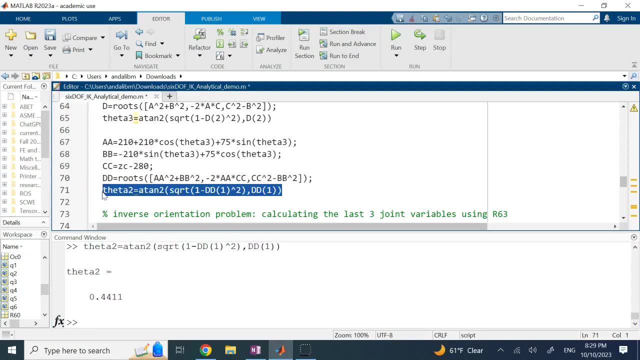 0.5.. 0.5, of course, with a negative number. Okay, If we use d, d, number 1, okay, and we did that, then we get 0.44.. So you might say: well, why didn't you get negative 0.5?? 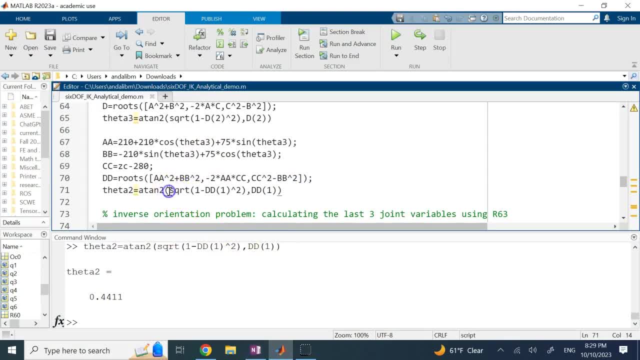 Because remember this equation here: when I say square root of this in general, it's positive and negative. square root of that right Sine is positive, negative. Square root of cosine 1 minus cosine squared, So this one is what. 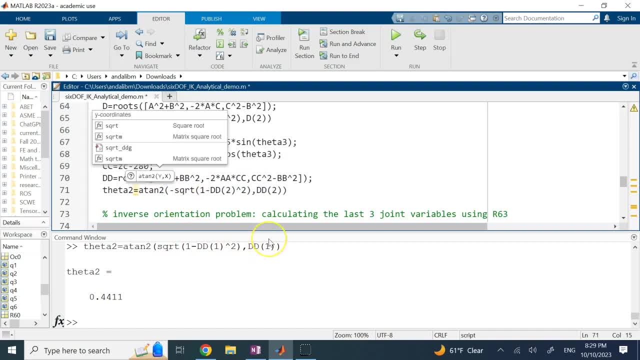 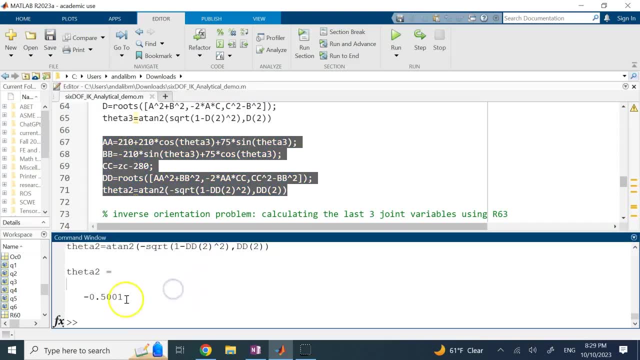 It could be positive square root, or it could be what Negative square root, And in this case this solution is the negative one. So if I do it again, you see that theta 2 is negative 0.5,, which is exactly this solution here. 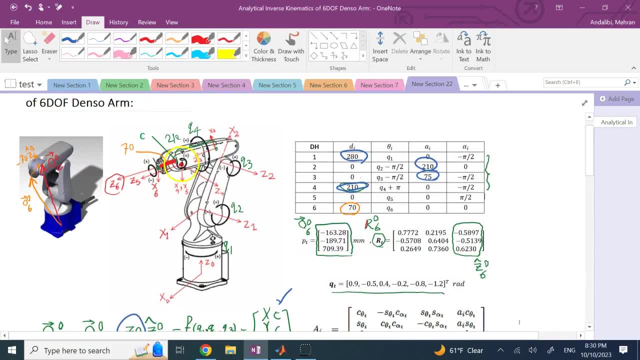 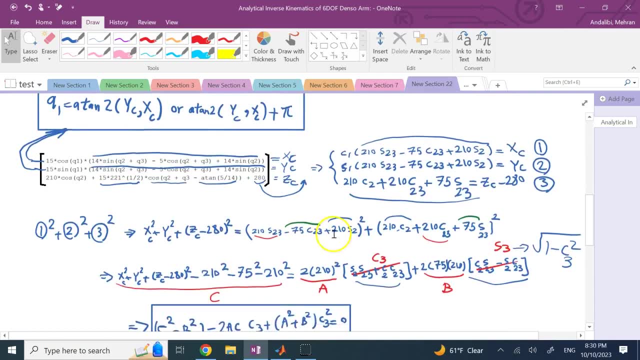 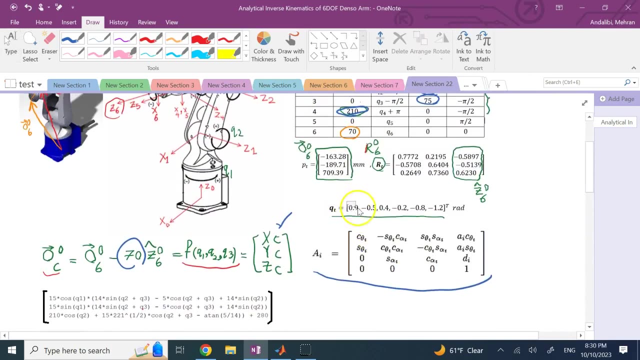 So so far, by calculating the risk position and saying that it's just a function Of the first three variables, I could find solutions for Q1,, Q2, and Q3.. And you see that I could get these three numbers. 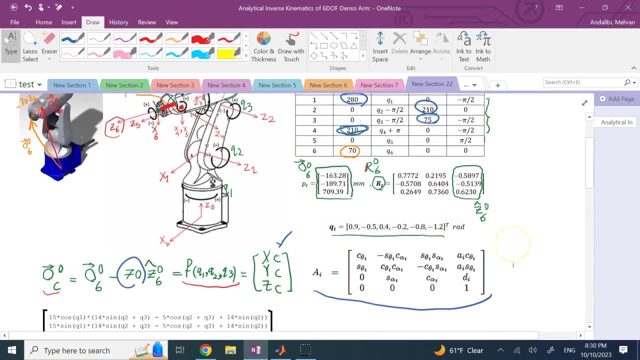 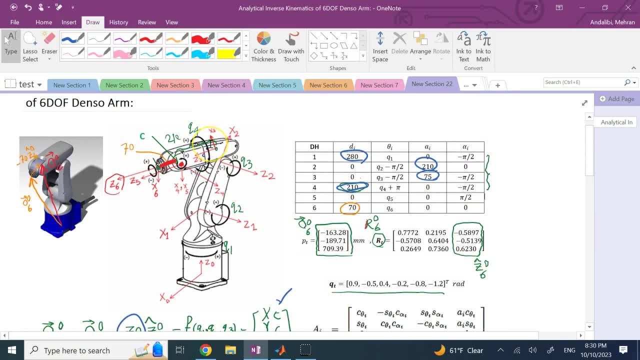 Now you might say: well, how do you get the last three joints? Well, let me show you. This time I look at the orientation of the end effector with respect to frame 3.. Orientation of the end effector R of frame 6, with respect to frame 3.. 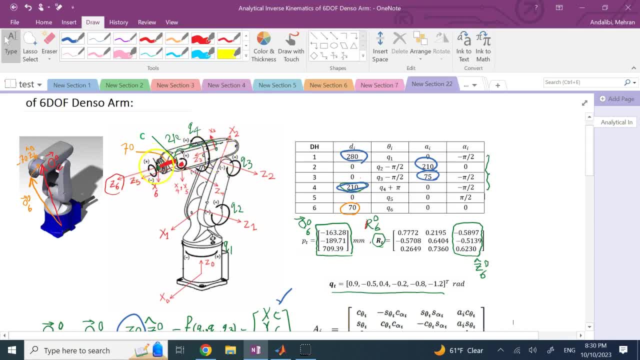 R of 6 and 3.. And this orientation of the end effector in frame 3 is only a function of what The last three variables right. So if the first three were in charge of the position of this wrist, the last three variables. 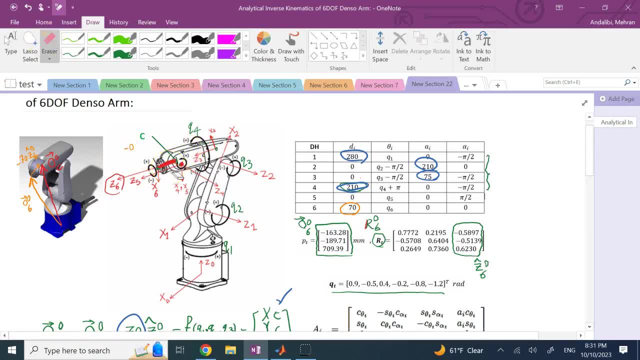 which is basically what. Let me do a little bit of cleaning here, Which is Is basically Q4, this Q here, which is Q5, and this Q here, which is Q6.. These last three Qs will determine what. 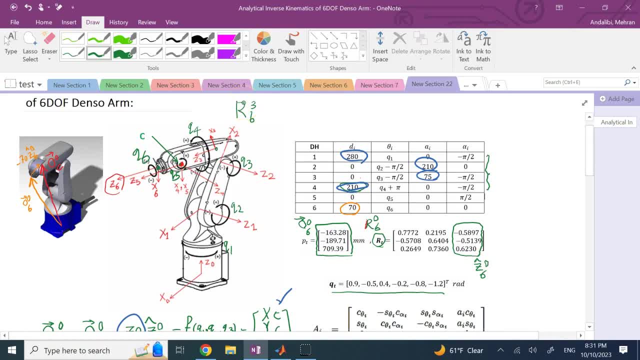 R of 6 with respect to 3.. Not 6 with respect to 0, because for 6 with respect to 0,, all six variables have a role. But for 6 with respect to 3, this is only a function of what. 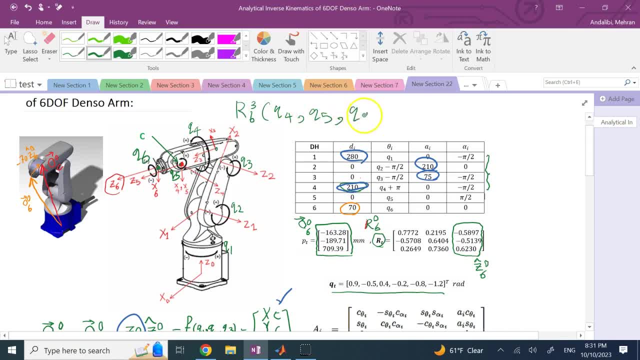 Q4 and Q5.. Q5 and what Q6.. It's just a function of those three joint variables. So you might say: how do I calculate this R of 6 with respect to 3?? Well, you know that if I multiply R of 3 with respect to 0 by R of 6 with respect to 3,. 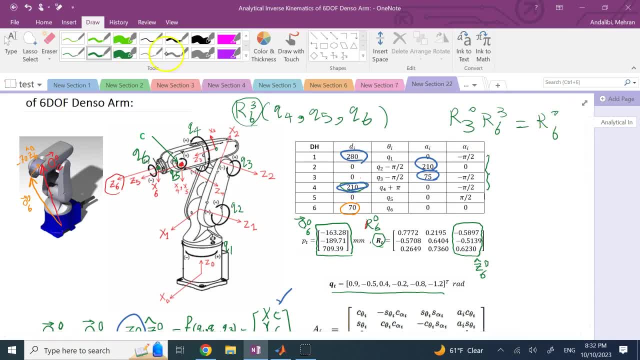 I will get R of 6 with respect to 0.. Well, this R of 6 with respect to 0 is given to me. Okay, That's a part of the inverse kinematics inputs. How do I get R of 3 with respect to 0?? 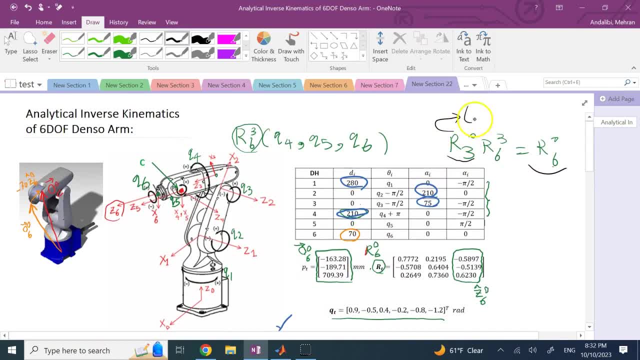 Well, R of 3 with respect to 0 is only a function of what The first three joint variables, of course. Right, So it's just the function of these three. Now that I have calculated these three, I should be able to calculate this R of 3 with respect to 0. 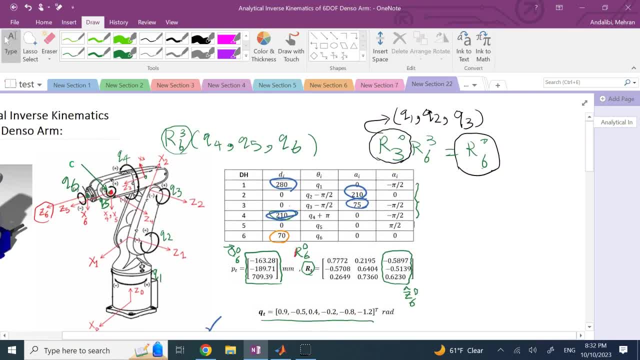 Once I have that, and I have the right-hand side, all it takes is to take the inverse of this, multiply, Multiply it by R6, 0, and you know, inverse of that is the same as transpose of that- and get R of 6 with respect to 3, and this is what I'm doing down here. 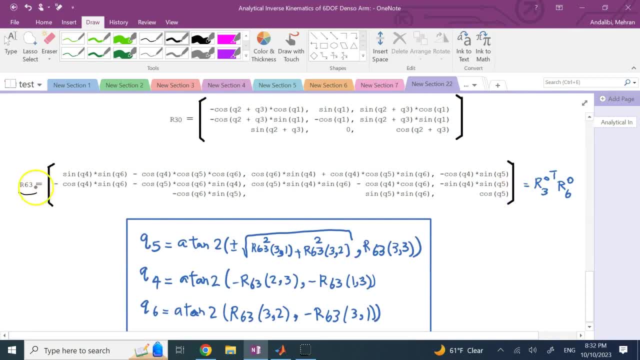 Okay, So this R of 6 with respect to 3 is R of 3 with respect to 0, transpose times R of 6 with respect to 0.. The question is: how do I get R of 3 with respect to 0?? 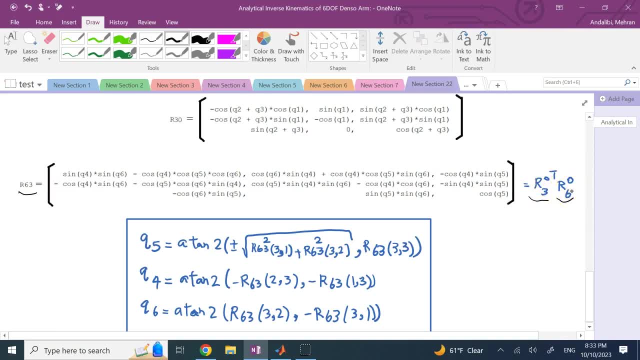 Because this one is just a bunch of numbers. Well, here this R of 3 with respect to 0, I can get it from T of 3 with respect to 0, which is basically A1 times A2 times A3,. 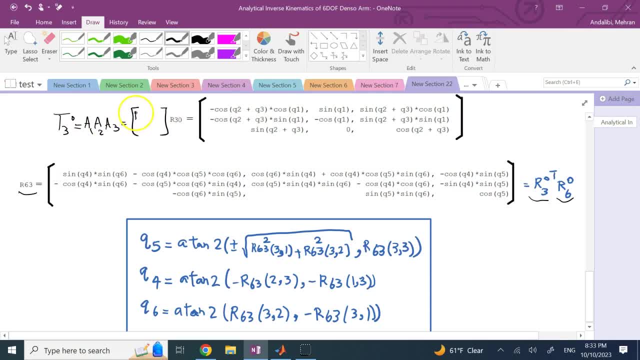 and it's a what? It's a 4 by 4 matrix where you have R of 3 with respect to 0,, where you have O of 3 with respect to 0, and then 0,, 0,, 0,, 1.. 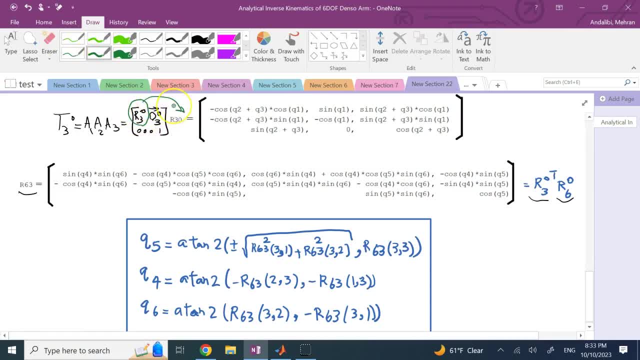 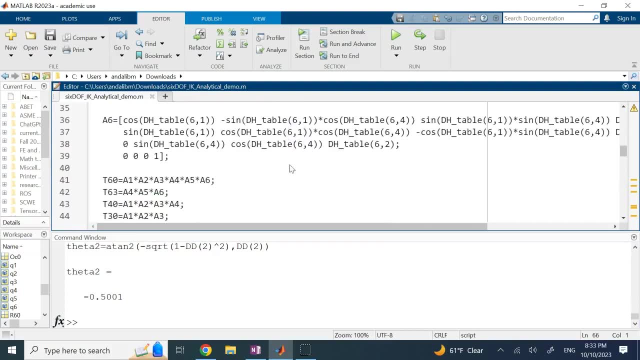 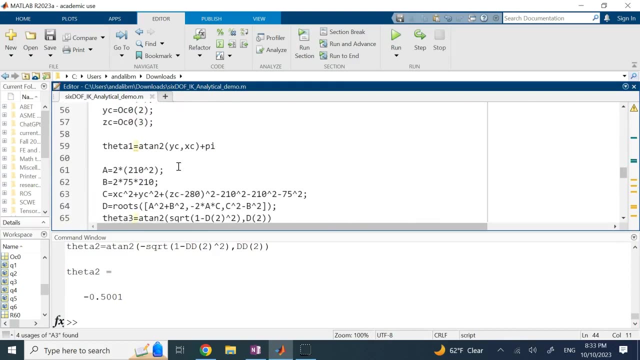 So if you look at this portion of it, that's what you want, And here I have calculated T of 3 and 0 symbolically. as you can see up here I calculated it. and then I look at the 3 by 3 minor part of it on the top. 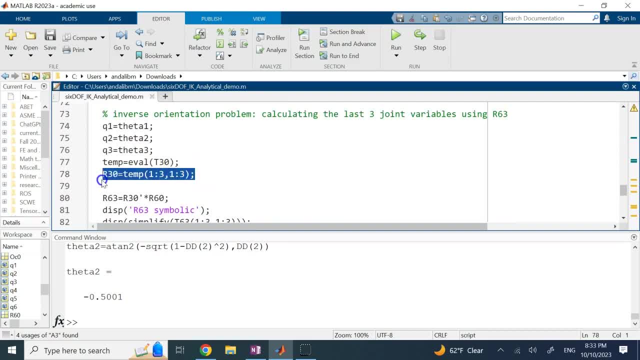 which is basically this part here. So what I do is the theta 1,, 2, and 3 that I found, I pass them to Q1,, Q2, and Q3, and then I put them together. then i evaluate t of three with respect to zero. so that gives me r of three with respect to zero. 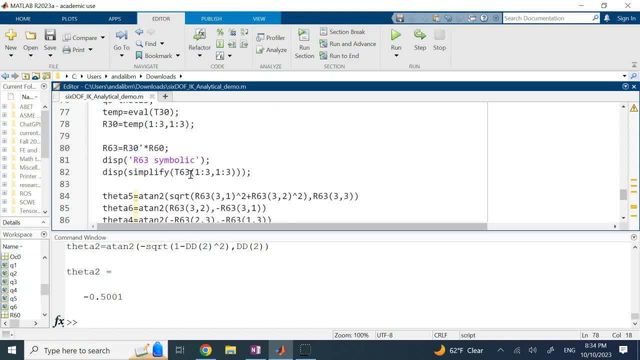 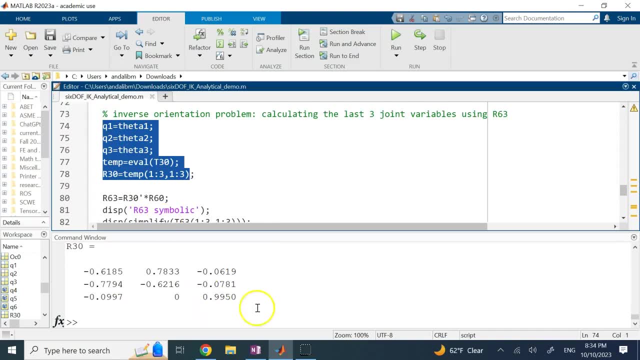 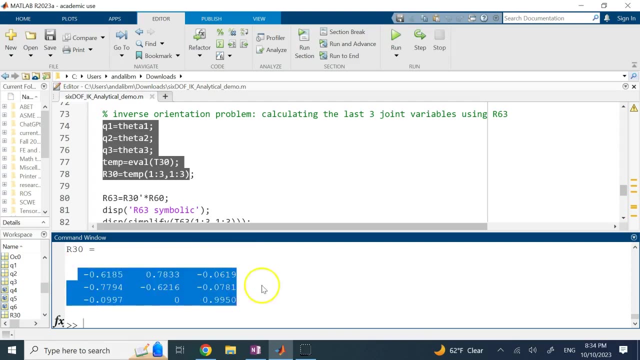 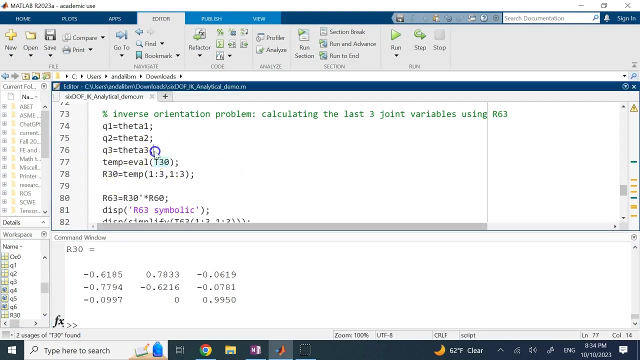 as a bunch of numbers. okay, it gives me those as a bunch of numbers. so here, look you see, this is r of three with respect to zero. as you can see, it's what it's: a bunch of numbers, because i know q1, q2 and q3 and i have evaluated my t of three with respect to zero using the three q123 that i 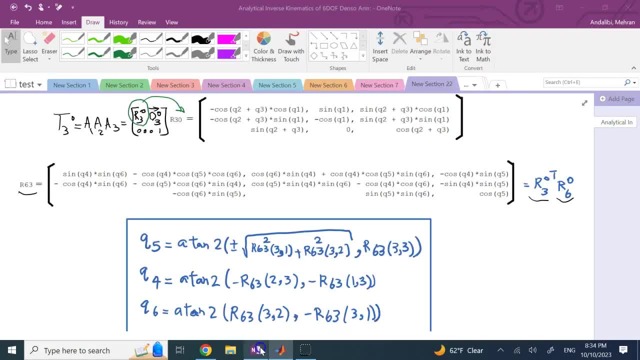 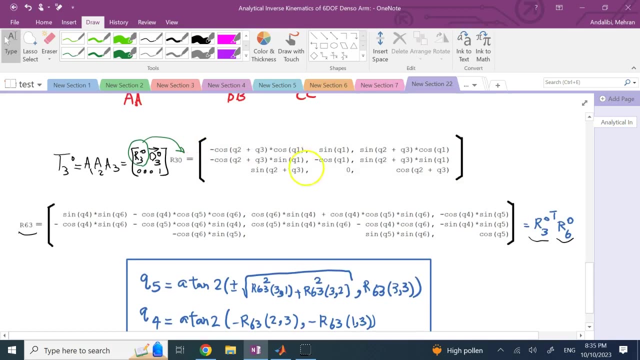 found. so now this is a number r of six with respect to zero is a bunch of numbers. so when i multiply together on the right hand side, i just get a bunch of numbers. now that thing- and, by the way, this is the formula, if you want it symbolically- this is the symbolic of t of three with respect to 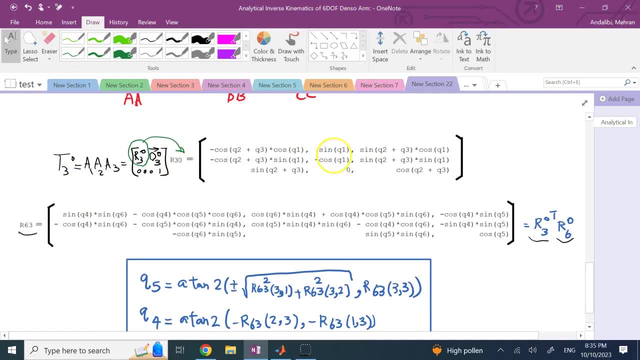 zero. okay, this is uh r of three with respect to zero and, as you can see, this r of three with respect to zero is only a function of q2, q3 and what q1 which i told you up here. okay, you see, i told you it's. 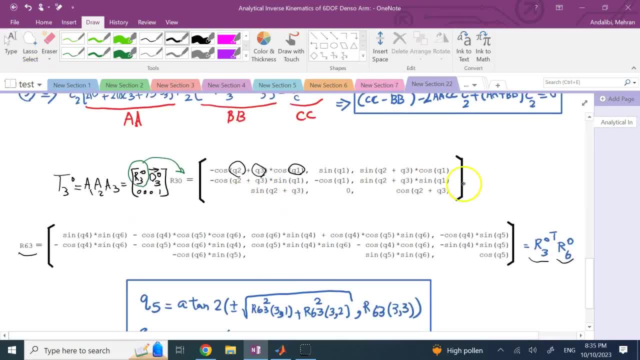 just a function of the first three, and of course it is. and these are those functions, but right now all i want is just a bunch of numbers. uh, well, what i want is just to plug q123 into these formulas. get this one good. so that is equal to r of six with respect to three. now the question is: 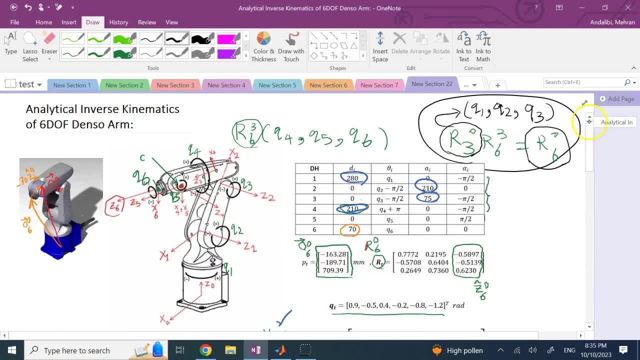 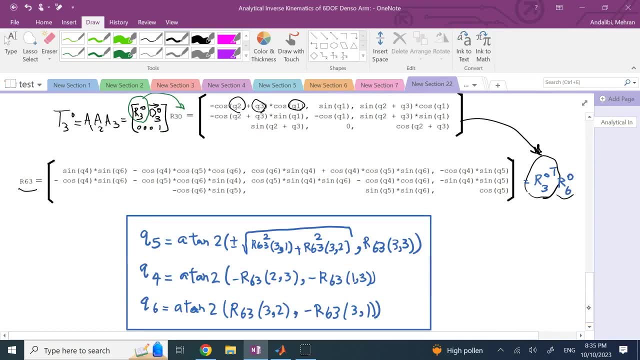 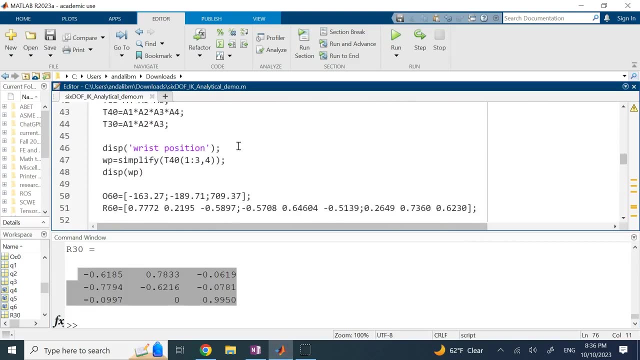 as i told you, r of six with respect to three is only a function of what, the last three joint variables. well, what kind of function? well, here i did it symbolically again, as you can see. i multiplied a, four, five and six together and i got what i got: t of six in. 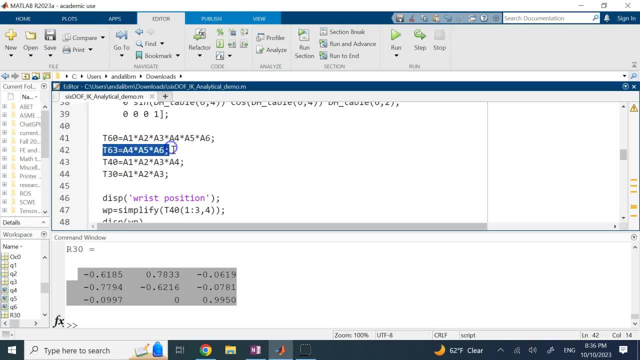 three and this is a symbolic function right now because i don't have a number for q- four, five and six. so this is a symbolic matrix and down here i am showing you that symbolic matrix. using the simplify command, i'm showing the rotation part of it, r of six in three. so look here. 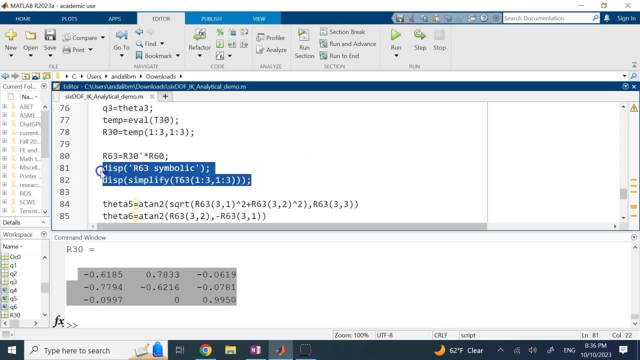 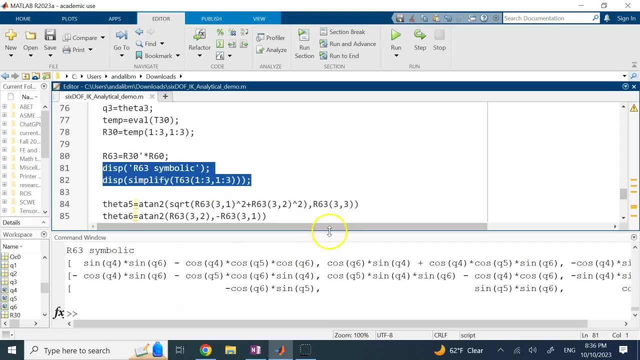 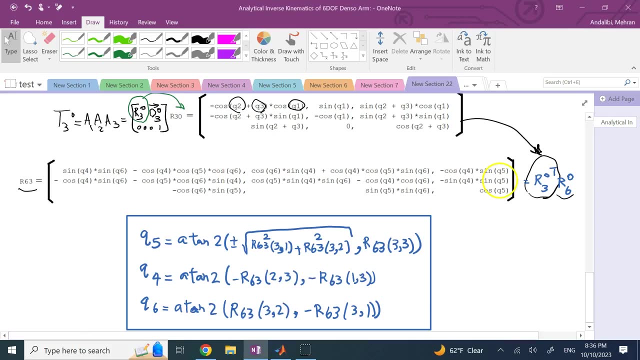 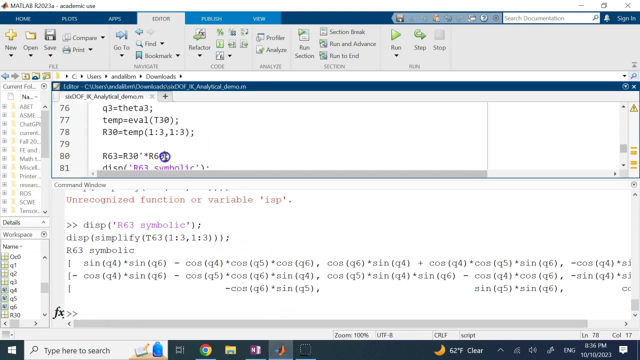 i uh get my symbolic part, which is this, and yeah, sorry here. so this is the r of six in three symbolic, which i copied it for you here, and the right hand side, which is r of three, zero, transpose r of six zero is what i have up here for you, this one, so that symbolic matrix should be equal to what to this? 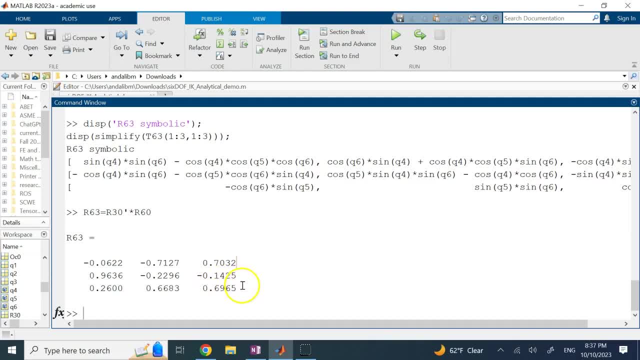 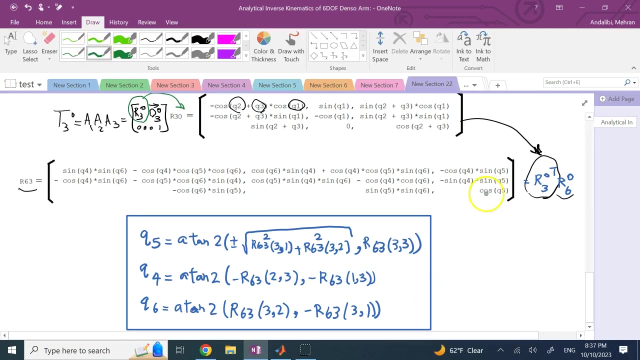 numerical matrix. and the question is, as you can see, it's only a function of the first three joint variables. so the right hand side shows all of the other joint variables in row one and half. so I and we can do this one sheet here at the first and I show you that theεια equation. 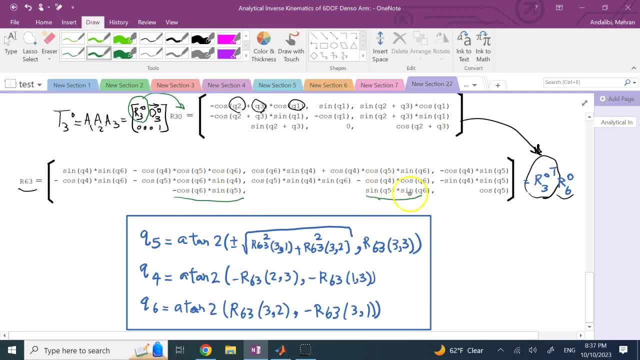 and the real thing on the명이 members is b? i to the i a. from this, studying the, it's going to be sine q5 squared times parentheses- sine q6 squared plus cosine q6 squared, which is 1, so it's just going to be sine q5 squared if I take a square root, which is this one. 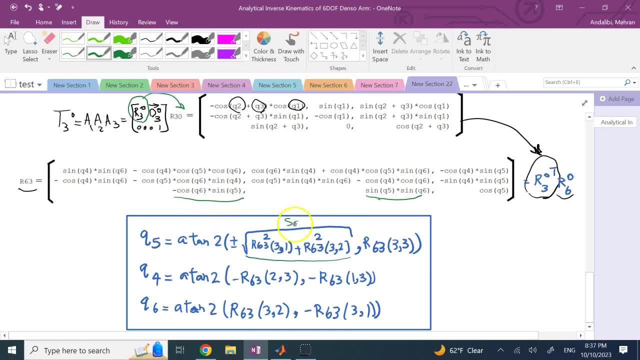 this is just going to be what sine of q5, and element 3, 3, which is this guy, is what cosine of q5. and if I pass sine q5 and cosine q5 to r tangent 2, that gives me what q5. now here, of course, 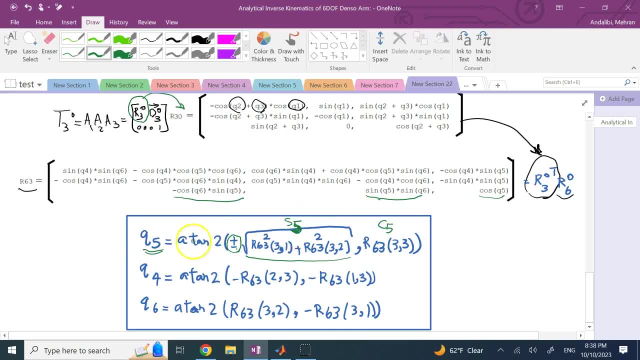 I have to use positive and negative to get sine 5. so that's another two solutions then for q4. what do I do? well, I look at these two elements here. if you can see, the elements are sine q4 and cosine q4, which I can pass to the r tangent command. but there is an extra negative. 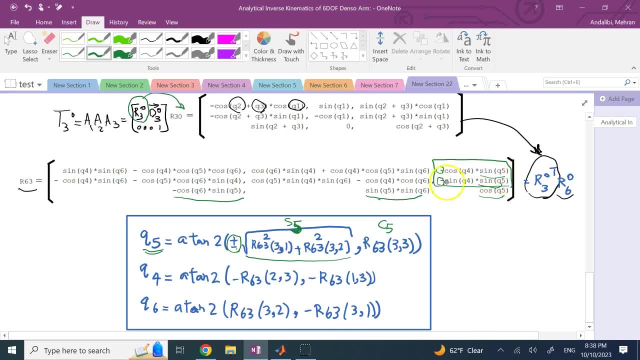 the sine q5, which is coming in both it's. there is no problem with that. but I need to multiply both of them by a negative, and that's what I'm doing here. right, element 2, 3, which is this one. element 1, 3, which is that one that becomes positive sine q4, sine q5 and positive cosine q4. 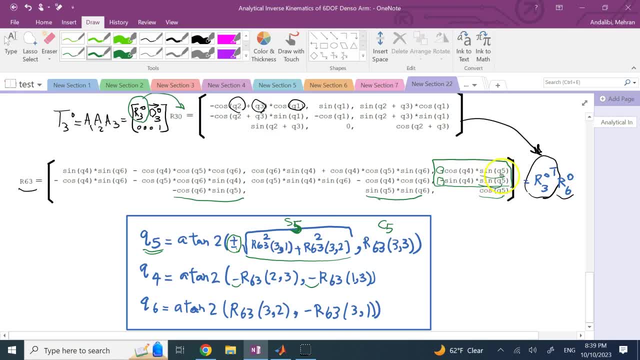 sine q5. again this erg, McMaster, constant sine q5 which is multiplied by both of them. it's not going to change anything. so I just pass those two elements with a negative and that gives me q4. and then I come back to these two and these two should give me what q6, because, again you see, sine q5 is multiplied to both of. 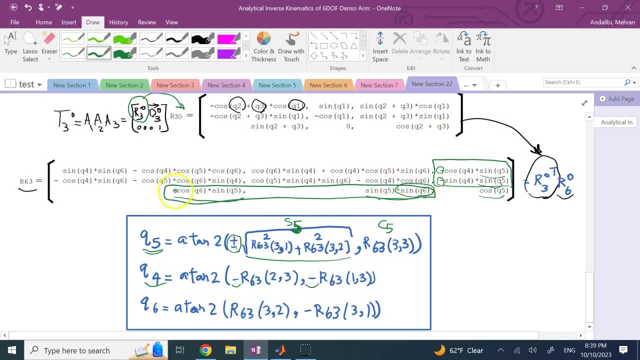 them. so I pass this sine q6 as the first one and then, to get rid of that negative, I multiply it by a negative, so that becomes cosine of q6 again, both of them multiplied by the same thing, which is not going to change the result. so I pass those two and that gives me what q6. and so, using these three, 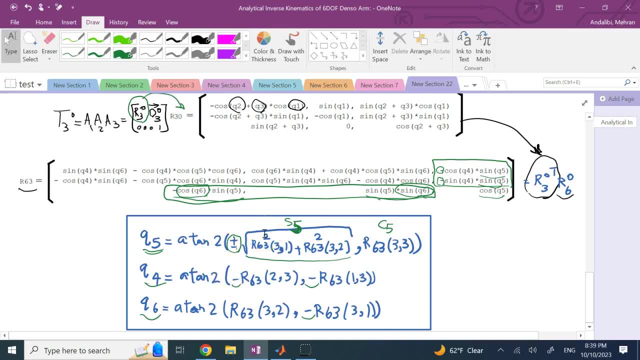 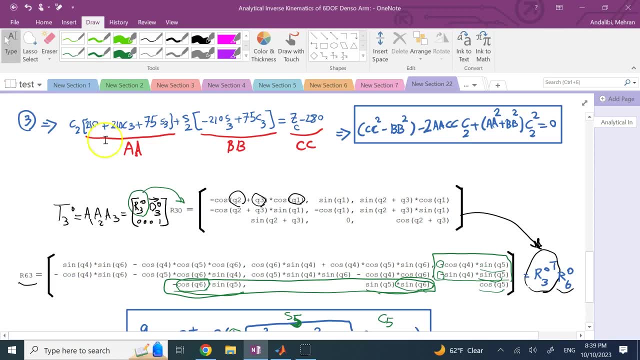 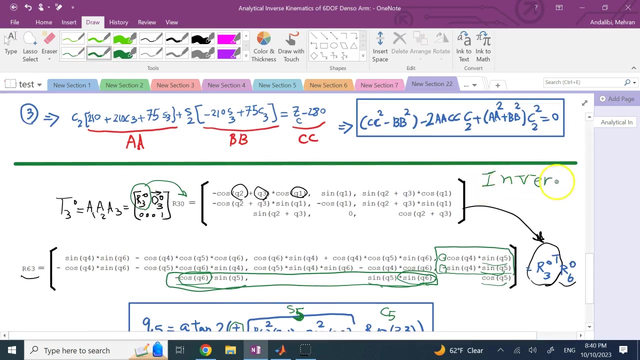 formulas. I should be able to get my q4, 5 & 6 and again this portion here, this portion that we basically used the orientation of frame 6 in frame 3, this part we call it what it has, a technical term, and we call it the inverse orientation problem. 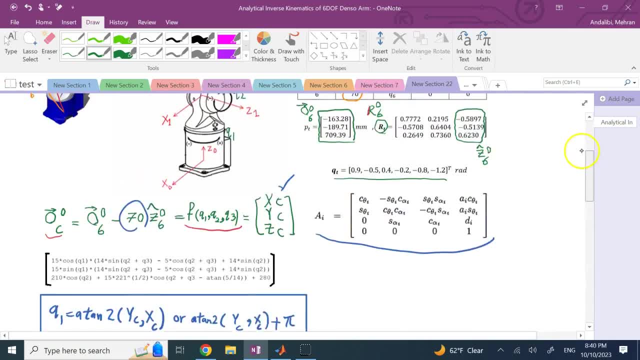 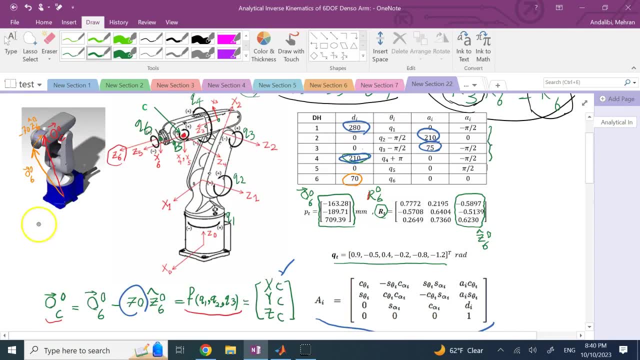 and the top part where we calculated the position of the center of the wrist, which was only a function of the first three variables, and using those I could find the first three variables. this part I call it what inverse position problem. so you see, instead of solving six equations and 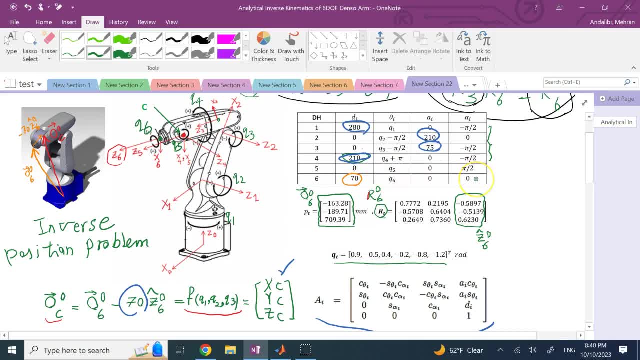 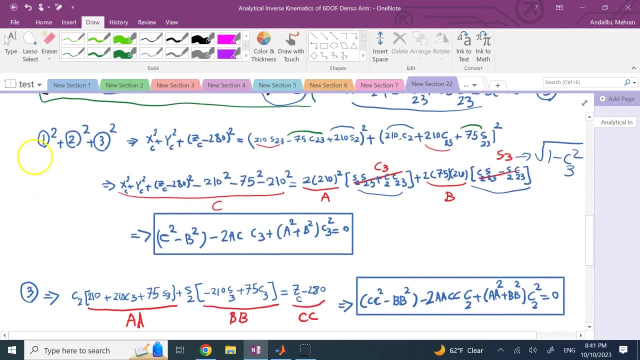 six unknowns which are highly non-linear in terms of q1, 2, 3, 4, 5, 6. instead of solving that, I broke it down into two sets of three problems. and what three unknowns. one of them was this one and the other one was this part here, and the other one was this one and the other one was this one. 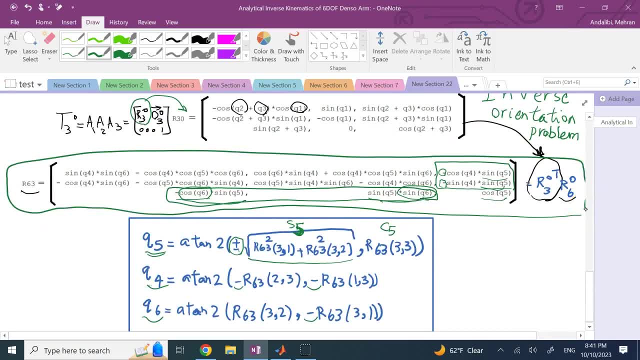 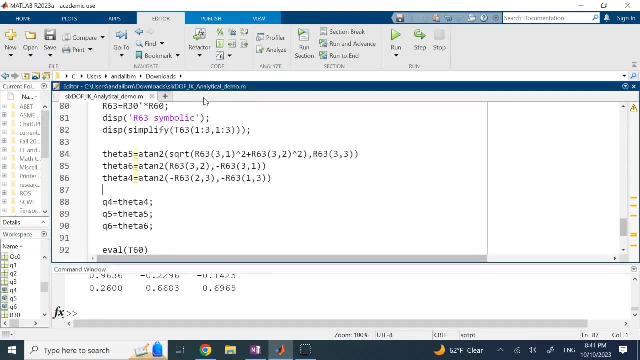 here and I could solve for all of my q's. so here let me run the whole program for you now, as you can see here, I have implemented those r-tangent formulas for 4, 5 & 6, and once I solve for them, I assign them to q4, 5 & 6. why? because I want to. 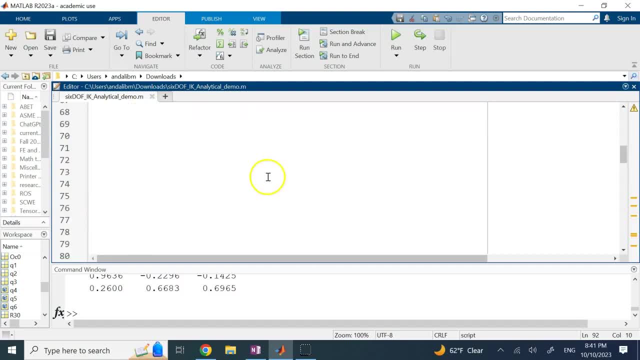 evaluate my symbolic function t of 6 and 0, which I calculated here on the top by multiplying all the a's together. I want to evaluate that symbolic function and I want to set it equal to what? to the transformation matrix, using the r60 and o60 which you see. 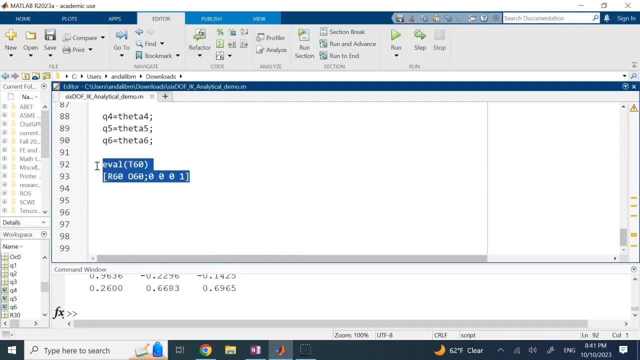 here I have put together. these two should be the same. so basically what I'm doing here, I'm plugging the ik solutions back into fk equations to see if they are correct, so if they can generate the same desired values when I plug them here into the symbolic equations, if they can generate. 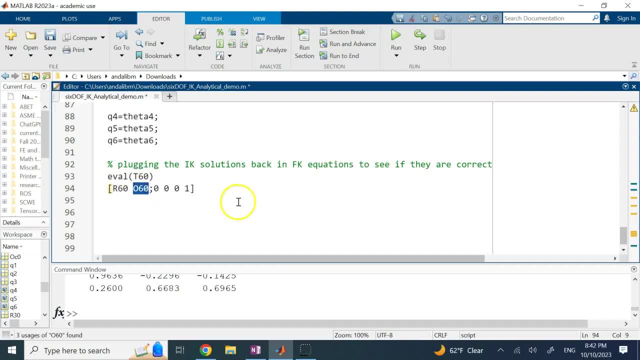 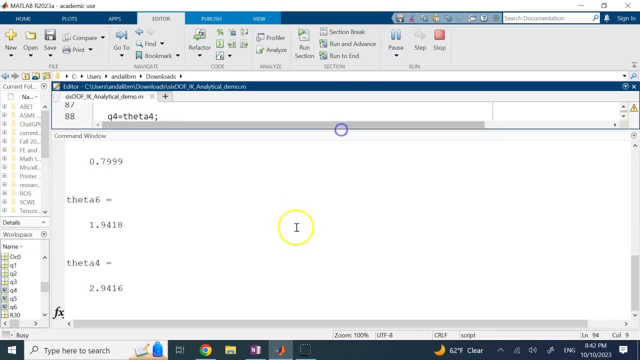 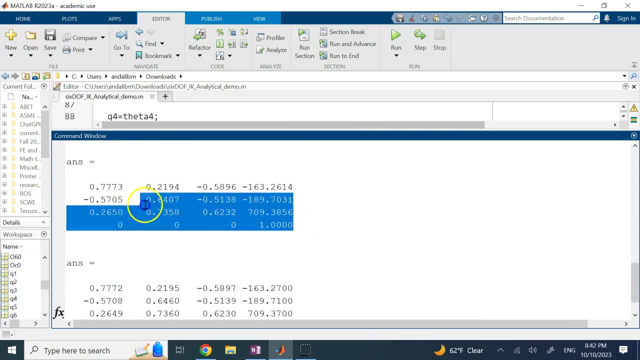 the same: desired values, desired rotation matrix and desired position. that means my solution is correct and let's do it here together. so there we go. this is the desired position and rotation matrix put together, and this is the result of plugging ik solutions into forward. k and you see they are what they are- identical, okay, except for some small. 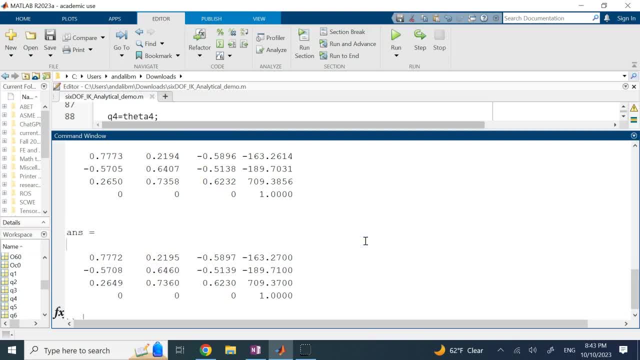 maybe 4. that's fourth decimal which can be due to rounding error or something. you see, the numbers are what equivalent? again, the robot animationvey Klein is going to come down here and say that if there is a true value to the within case of a basic alboразion matrix used by an English parameter, So you can apply this kind of a method because you can pretty easily do this using other way. you can put a success cow. however, if you do this in the function Nash implementation in the function Nash implementation, so that defy for your方ah is justU Shop. this is the result of plugging I ket solutions into 4 word k, so it's already. 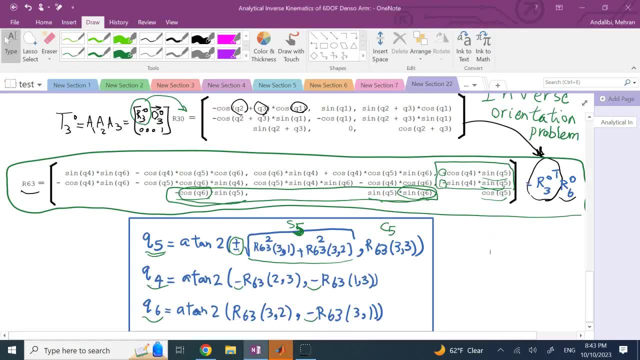 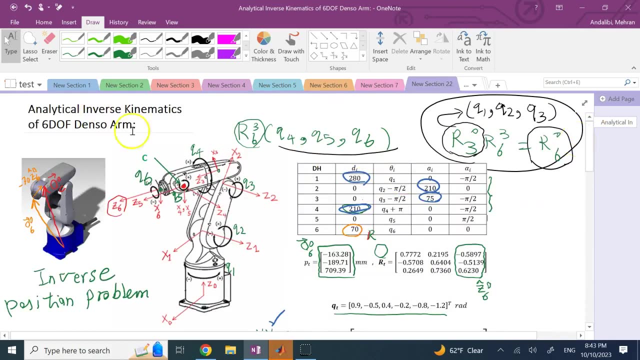 the robot has the inverse kinematics problem of that has 16 different solutions. has 16 different solutions in general and here we just focus on what one of these solutions which is provided here. but clearly you can see that it is working and we can solve this in ik of this robot. 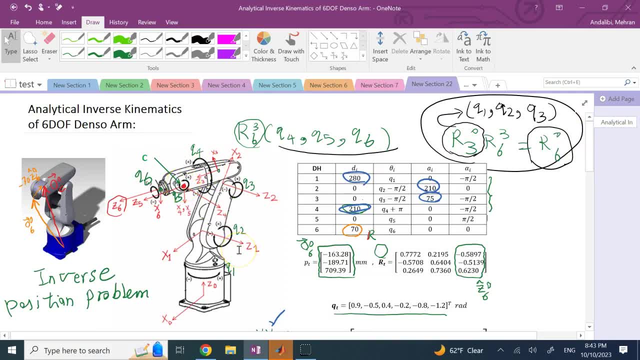 analytically, because it has a spherical wrist and it's only 60 of. hopefully, this video was useful to you and i'll see you in the next video. thank you.